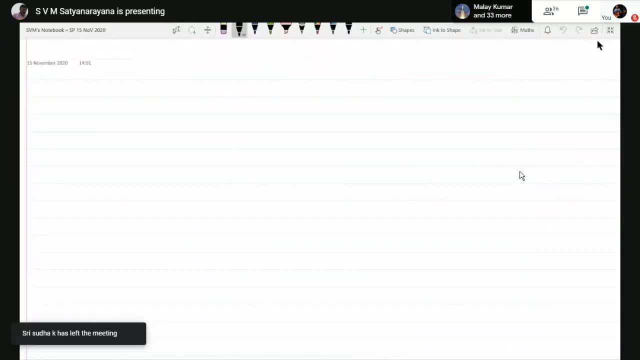 So let me just make. We will come back to some of classical applications of grand canonical ensemble and do them later, but let us go and look at quantum statistical intent. So here we are going to talk about So one of the important things that I will. 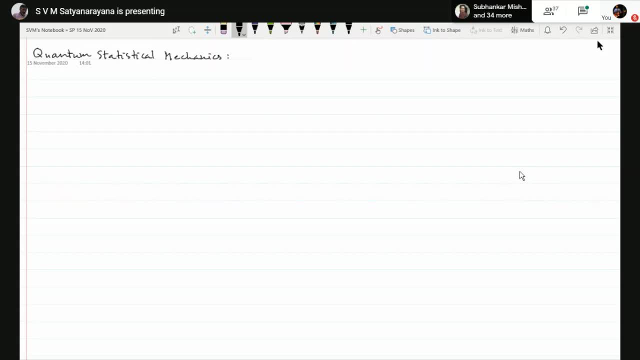 consider is that we are always going to consider non-linear, non-interacting system, Non-interacting system. So one of the advantage of non-interacting system is that you can use something called. In this case, we can use single particle, single particle energy. 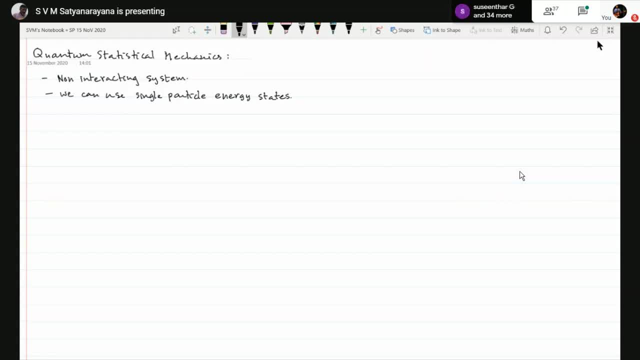 For example, let us say that, let us say there are n particles, n particles and these particles are non-interacting. Those are non-interacting, These are non-interacting. So now let me set the representation. So let us say that I have particle 1. 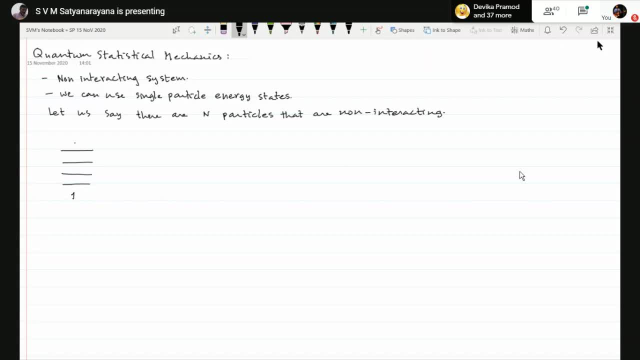 and I have certain energy levels for particle 1. There are infinitely many energy levels and particle 2 and that has got certain energy levels. There are also infinitely many in particle 3. It has its own energy levels And we update these energy levels by solving the quantum mechanical problem. 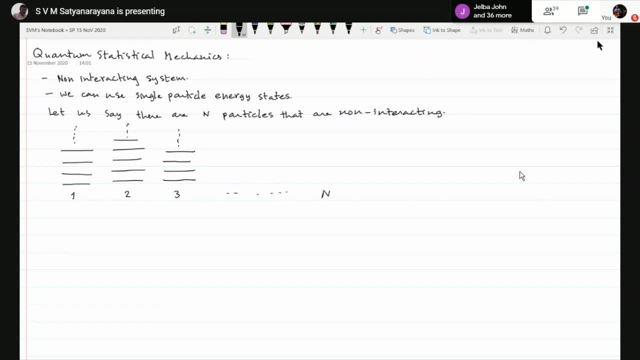 And like that I have some n particles- which has its own energy levels, So these are what we call as single particle energy stress. Now, if there is no interaction between them, the energy levels of one particle will be same as that of the energy levels. 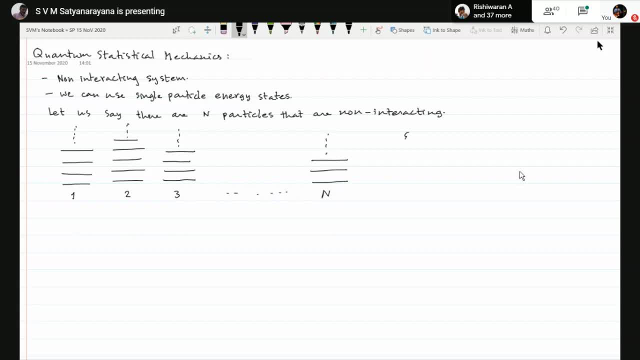 of the other particles. For example, if you consider, let us say, n particles, n particles in a box of volume, then we have the energy levels, as we can call it as n1, n2,. n3 is equal to h bar square. 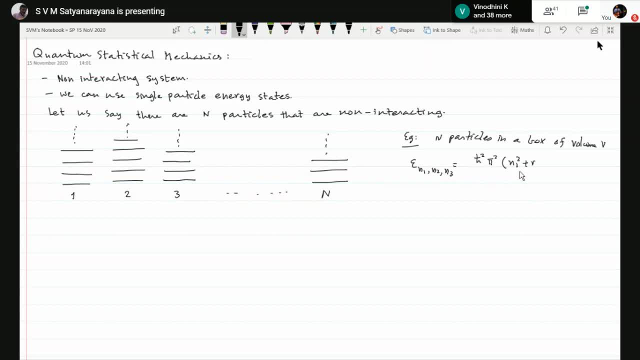 pi square into n1 square plus n2 square plus n3 square, divided by twice n v to the power 3.. So these are the energy levels of particle in a box. because these particles are non-interacting, Each of the particles has the same set of energy levels. 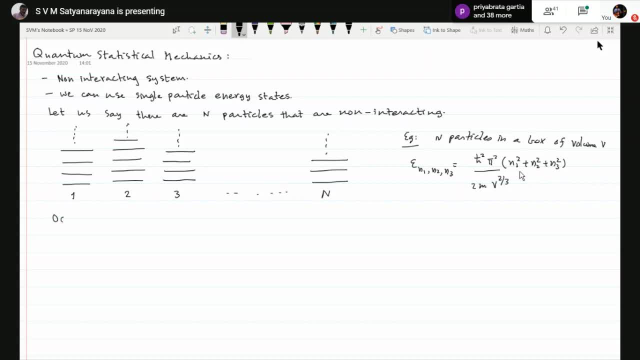 Now we have something called occupation number representation, Occupation number representation. So this representation is what we will use and what is the representation? Let us say I have epsilon 0,, epsilon 1,, epsilon 2,, etc. These are my energy levels. How many of them? 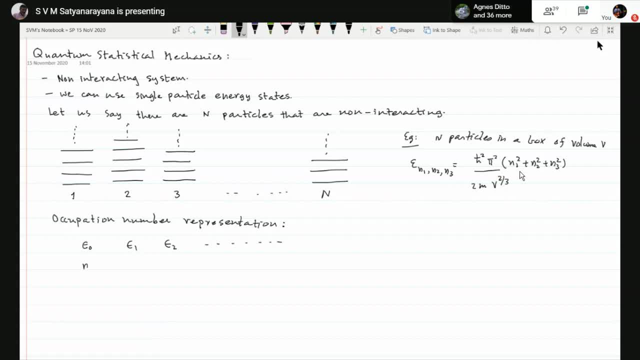 Let us say there are n0 number of them. n0 of the particles are in the ground state and n1 of the particles are in the perspective state and n2 of them are in the ground state And these numbers are called occupation numbers. 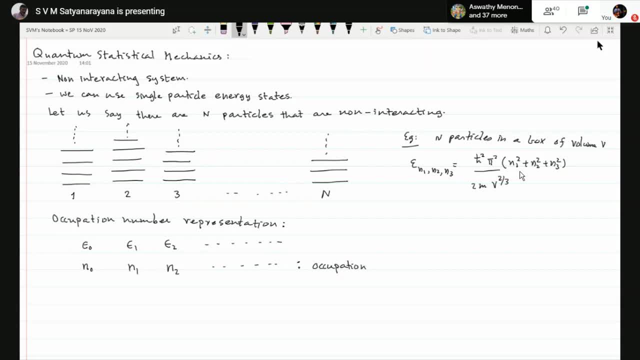 What is occupation number? And once these numbers are fixed, this particular number, we define it as one particular mode. But there is a constraint on this. The constraints are, let us say, 1,, 2,, 3,, 4,, 5,, 6,, 7,, 8,, 9,, 10,, 11,, 12,, 13,, 14,, 15,, 16,, 17,. 18,, 19,, 20,, 21,, 22,, 23,, 24,, 25,, 26,, 27,, 28,, 29,, 30,, 31,, 32,, 33,, 34,, 35,, 36,, 37,, 38,, 39,. 40,, 41,, 42,, 43,, 44,, 44,, 45,, 46,, 47,, 49,, 50,, 51,, 52,, 53,, 54,, 55,, 56,, 57,, 61,, 62,, 62,. 62,, 62,, 63,, 62,, 63,, 62,, 62,, 62,, 63,, 62,, 62,, 63,, 62,, 62,, 64,, 64,, 65,, 67,, 67,, 68,, 68,. 69,, 68,, 69,, 70,, 8,, 89,, 90,, 90,, 90, 90.. And sum over j mj would be equal to the total number of particles And sum over j mj times epsilon j is equal to average energy of the particles. 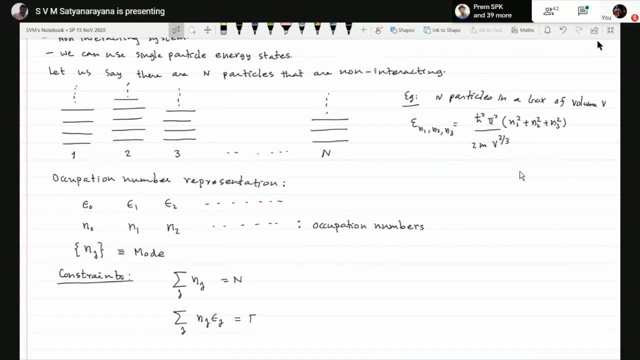 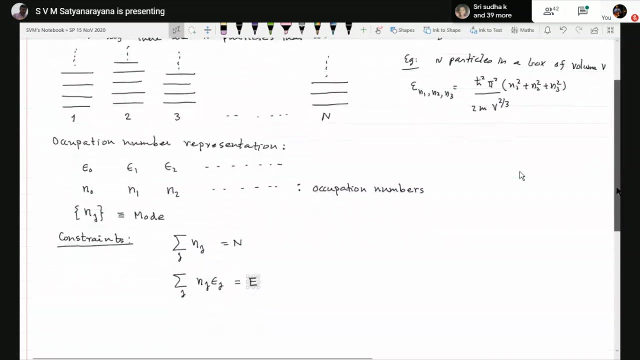 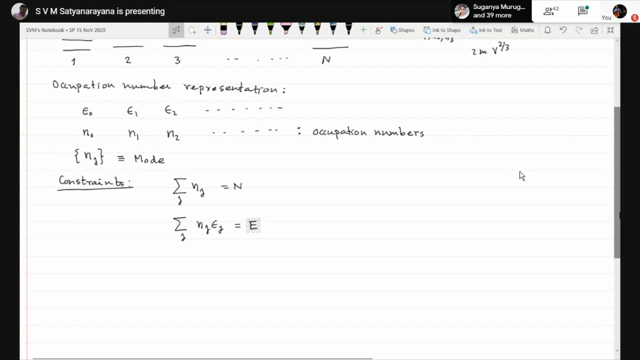 Now these are the two constraints- that the occupation numbers have to be applied. Now, these are the two constraints that the activation numbers have to satisfy, Sir, for photon gas. it doesn't satisfy for photon gas right now. I am keeping it very specific, So this is a general thing. So now, what happens is that, suppose, if you are, 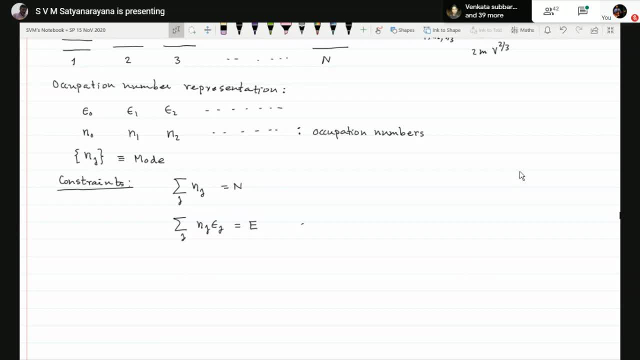 interested in writing down a kind of a grand canonical partition function. So suppose we have, let us say, for a given configuration, configuration of a mode. So this is the configuration of a mode. Okay, So we have an NK. Okay, So you know, this energy is given by this energy is given. 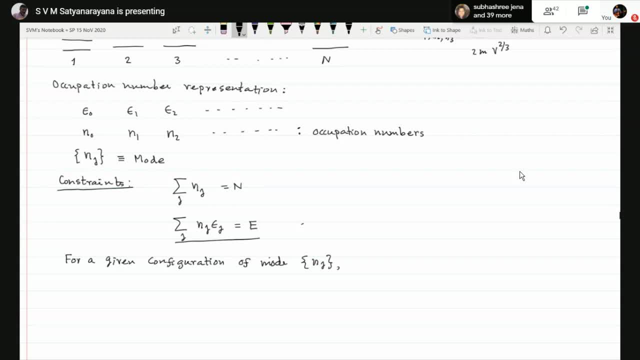 by this, Entire number of particles are given by this, So we have energy or from this component. So now suppose, if you are interested in writing down the grand canonical partition function, so we can write grand canonical partition function. so let me write this as Q times Q of beta, V comma. 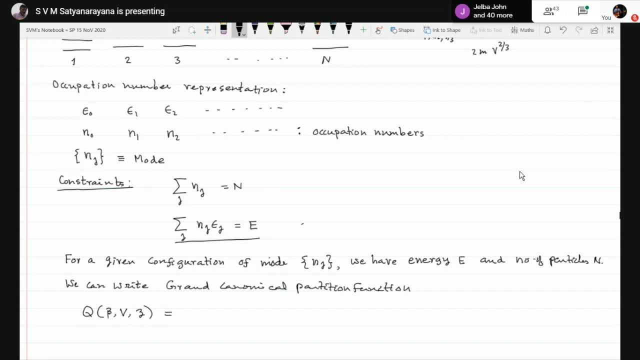 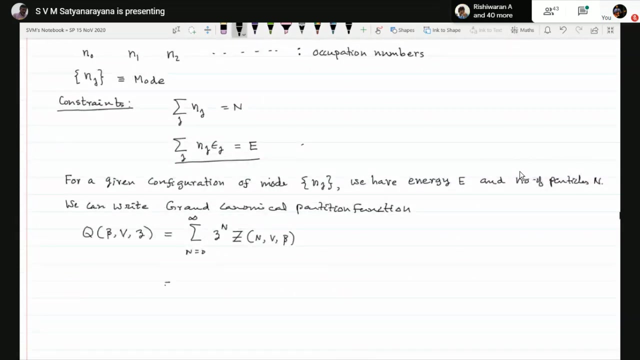 of the fugacity z, as sum over n is equal to 0, to infinity z, to the power n into, of course, the canonical partition function, because that is what we have in terms of that is essentially canonical partition function of n, V. Now canonical partition function for n number of particles can be written in the following: 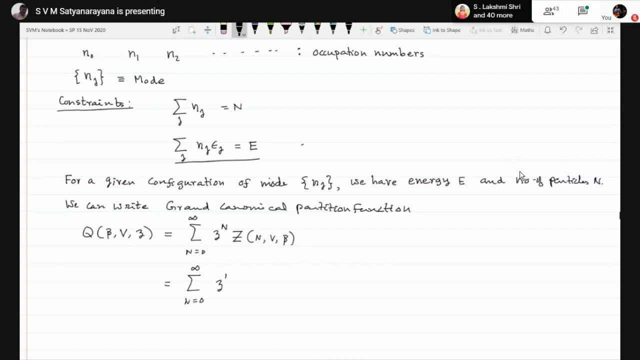 pattern. So this is equal to sum over n, is equal to 0, to infinity z, to the power n, and now I have to take sum over all these possible nodes. that means a kind of a power set, and this sum is 1.. 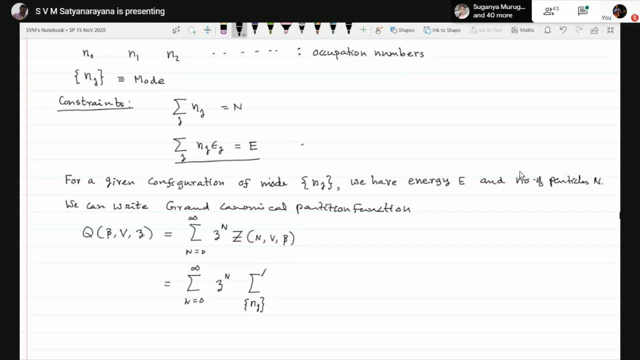 is constrained by the constraint. that sum over j, n. j is equal to n is the constraint. and then I have e to the power minus eta into the energy. energy is n: 0 epsilon 0, n, 1 epsilon 1.. So this is canonical partition function. So this is something which we have to do. 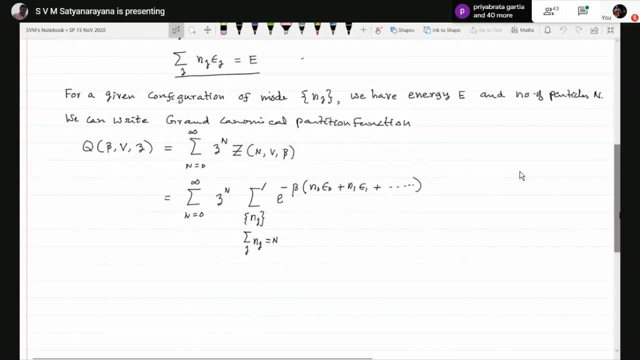 with it for the value. Now this constraint summation can be made into an unconstrained summation. So note the following result. note that suppose if I have sum over n is equal to 0,, 3 and sum over n is equal to 3.. 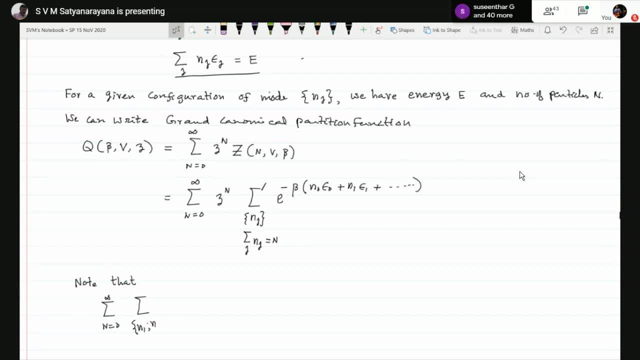 So now what do I do? I will write a constant summation of n equal to 0 to 1, and I will Let us say: n 1 comma n 2, sum over n 1 comma n 2, with a constraint that n 1 plus n 2 is. 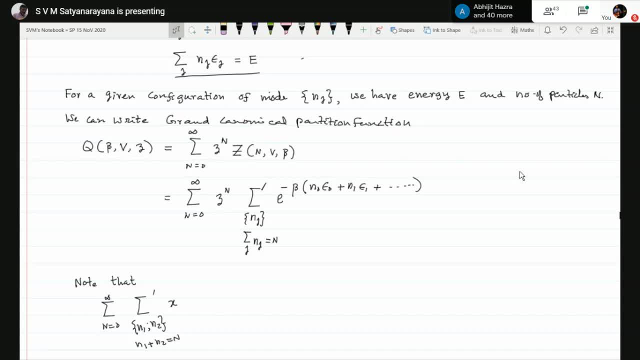 equal to n into some x to the power n 1 into y to the power n 2.. Let us say I have some information like this Now. this can be written as: sum over n 1 is equal to 0 to infinity x to the power n 1. This is an unconstrained sum over n 1, and sum over n 2 is equal to: 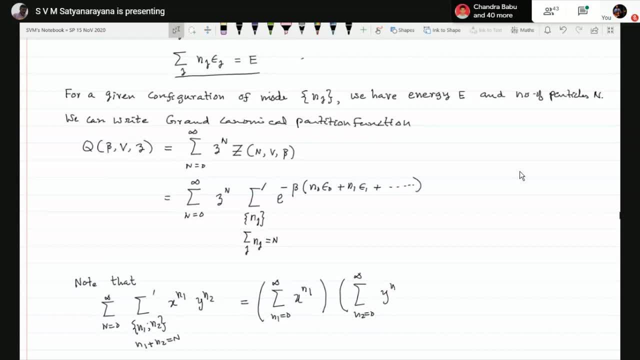 0 to infinity, y to the power n 2.. Both are unconstrained sum, So this is something that can be written Now. it is not very difficult to realize this. For example, let us try to evaluate left hand side. So if you take, n is equal to 0 and n 1 and n 2 has to be equal to 0. So let us 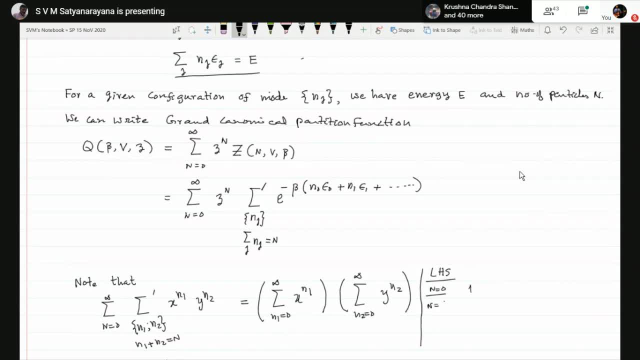 say n 1 is equal to 0 and n 2 has to be equal to 1.. Suppose, if you take n is equal to 1, n 1 can be 0 and n 2 can be 1, or n 2 can be 1 and n 1 can be 2.. That means you can have: 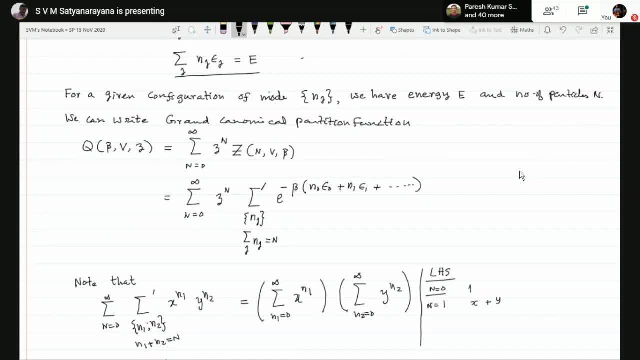 terms like x plus y. And now, if you take n is equal to 2, then you will have x square plus y, square plus x times y, and so on. So this is an unconstrained sum over n, 1.. So 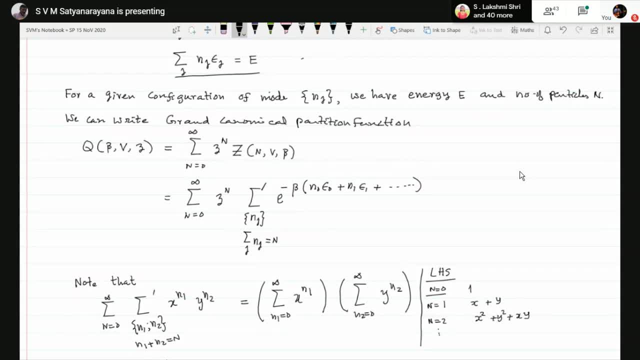 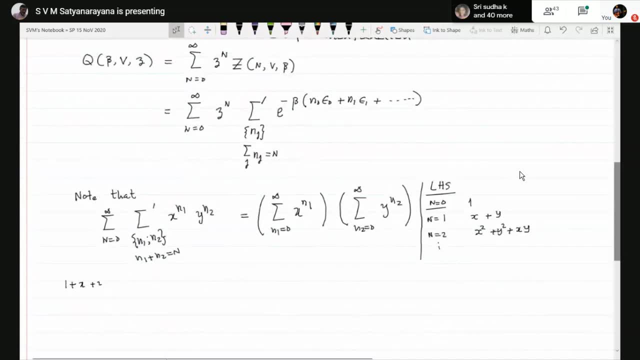 left hand side is going to be something like this: 1 plus x plus y plus x square, plus x, y plus y square, And so this is what is going to be. That is next you will have all cubic terms, that is, x cube, x square, y, x y square, y cube, and so on. 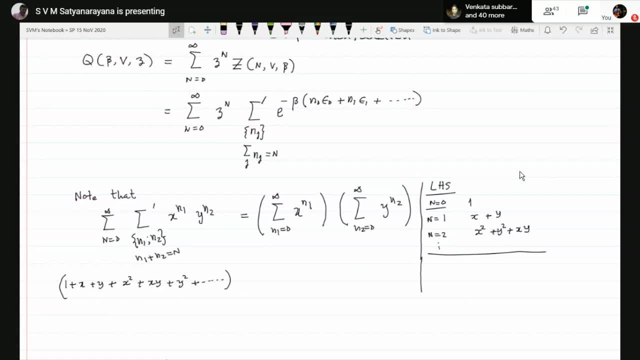 Now look at right hand side. right hand side is something like this: 1 plus x plus x square, etcetera, a product of this with 1 plus y plus y square. So look at first few terms. that is, 1 plus x plus y plus x square, plus x y plus y square. 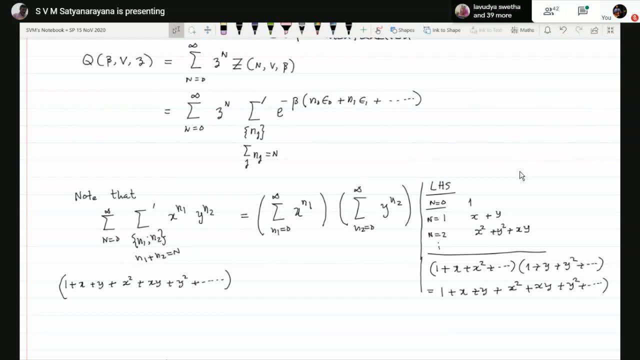 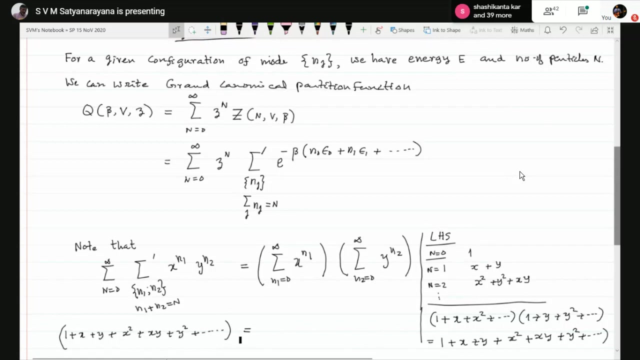 square, So you can see that term by term. this left hand side and right hand side are going to be same, So that way you can verify that this constraint sum on the left hand side can be written as a product of unconstrained summation. 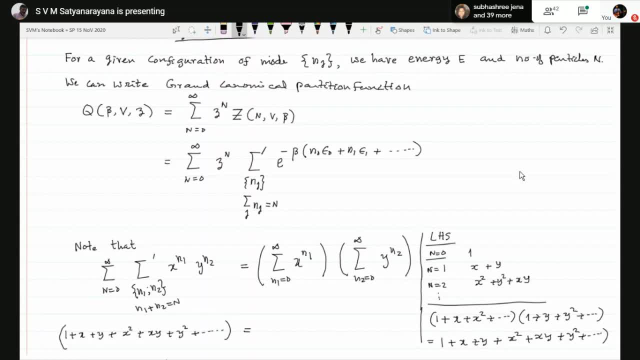 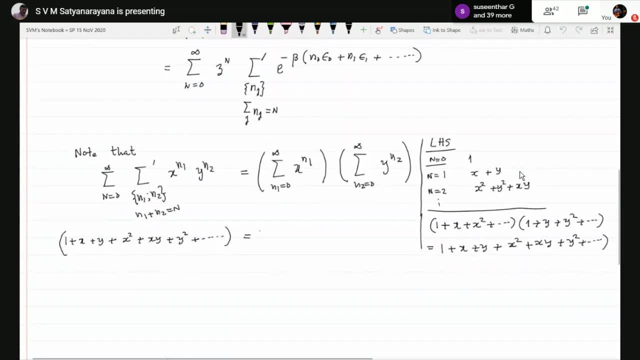 And this can be written even if you have a more than 2 industries. So this tells us that this is 2 square, y square, 3 y square. So, if you understand this mathematical equation, there are two largest equations, which are of the kinds: So the first of which is the Hess beautiful economic factor, such that he has said f acting on x, x, y, x plus x, y, t plus xx plus x, x times z, into 1 times x, 2, x, q times z, k, cos times dr plus x, t, I the one, and that is, flavors of the corresponding equations were: 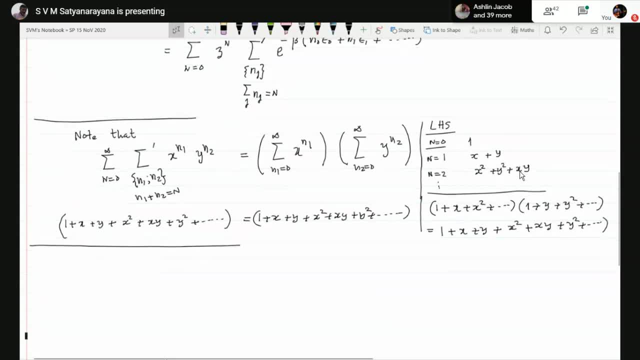 So if you understand this mathematical equation- there are two consistence numbers over here, because this is a very large displacement diagram- then the grand partition function now can be written as: note that: so we have this grand partition function. z is equal to- I can write down this: n is equal to 0, to infinity, this 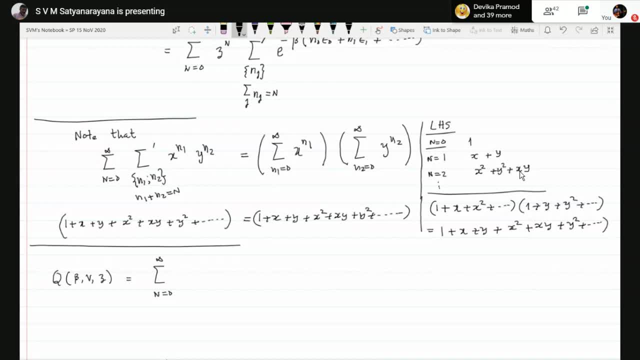 capital n is n1 plus n2 plus n3, right that is z of n0 plus n1 plus etcetera, into sum over these nj's. and it's a constraint that sum over the nj into 2 to the minus beta of n0, epsilon 0.. 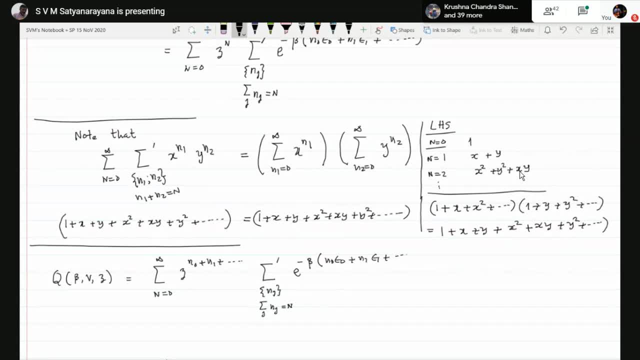 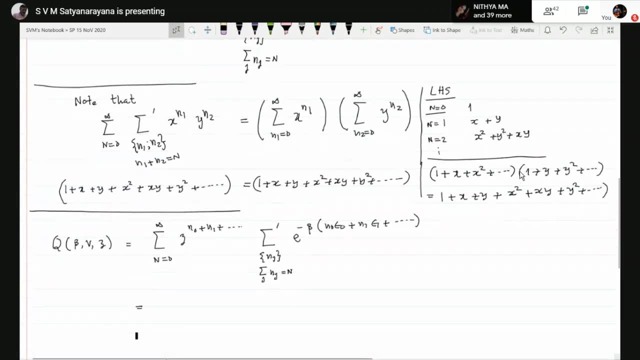 Now this can be now written by using the above mathematical equality. this can be written as: sum over n1 is equal to n0 is equal to 0 to infinity e to the minus beta epsilon 0 into z. So this is one term. then I write: the product sum over n1 is equal to 0 to infinity z, e to 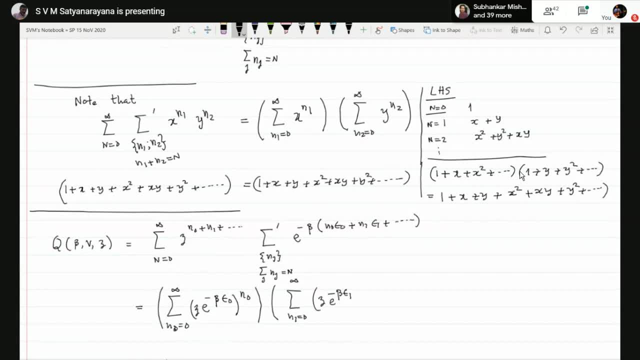 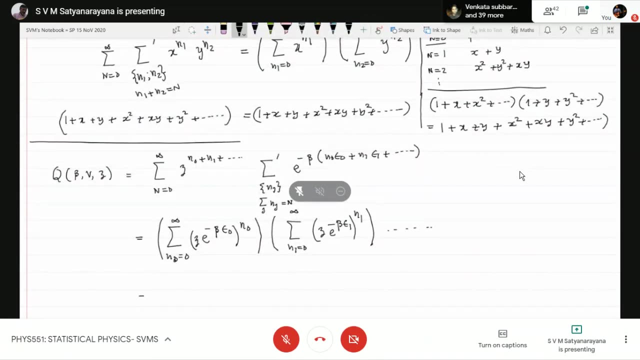 the minus beta epsilon 1, raise it to the power n1, and so on. I will have infinitely many such terms, but for every energy level there is one term, and I will have it into 2- to the minus beta value. Now this can be written in a short hand notation like this: which is called product, which is 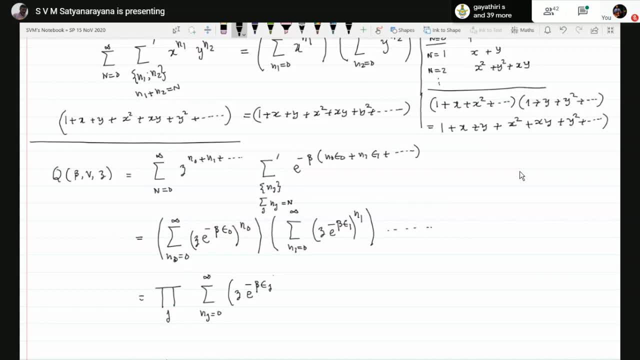 a symbol for product over j. sum over nj is equal as 0 to infinity. z e to the minus beta. epsilon j raise it to the power n, So Q beta is grand canonical partition function for a system of non-corruption. Now you can see that, this particular equation, you can see that this epsilon j, what are? 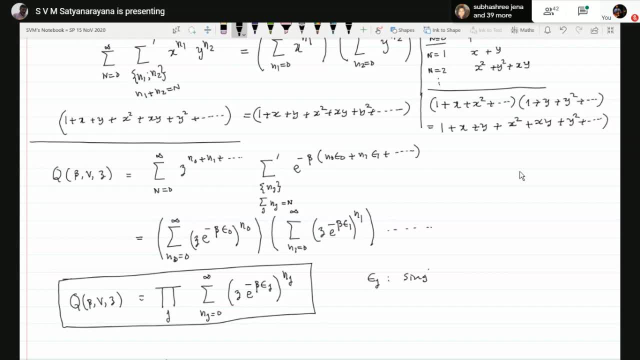 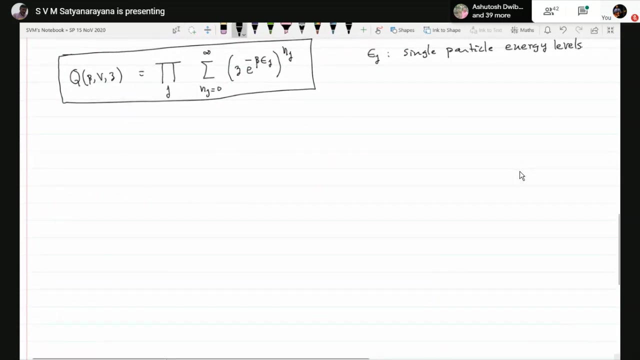 these epsilon j. These are single particle energy levels. single particle energy levels, So this expression. up to this we have been quite general. Now we cannot be general henceforth. We have to ask the question: what kind of these particles? 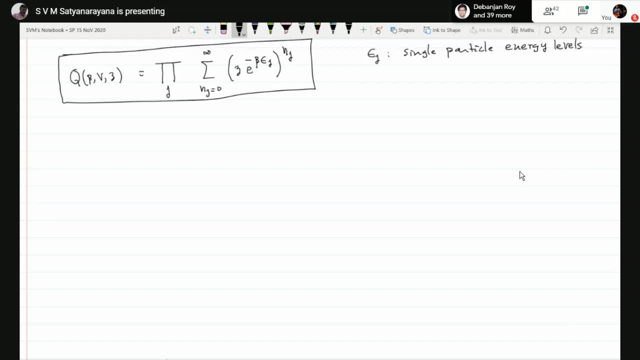 What kind of particles of particles. So in quantum statistics, based on the nature of particles, you have two distinct statistics. ok, Soif you have fermions, you have fermions. these areparticles, particles with half integral spin, half integral spin. So these are the particles with half integral. 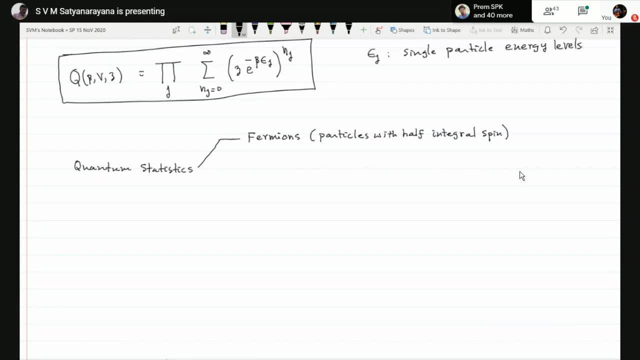 spin, then they their total wave function. their wave function must be anti-symmetric- anti-symmetric upon exchange any pair of particles. This implies that if you have an anti-symmetric particle, the particles, particles convey what is called how these fusion function. 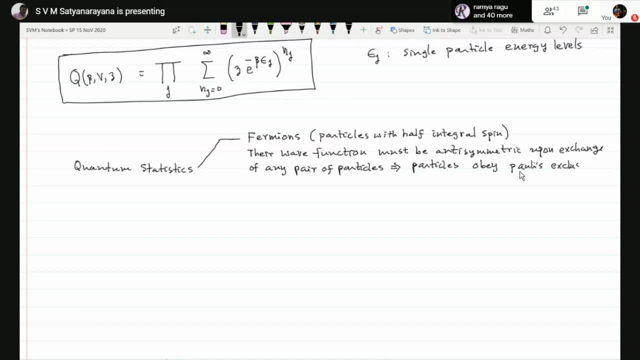 How these fusion function. This is called how these fusion function. So if you have a single particle, single particle means for any single particle, single particle energy state. The optimization number of the single particle energy state is different. Occupation number can be 0 or 1 and nothing else. 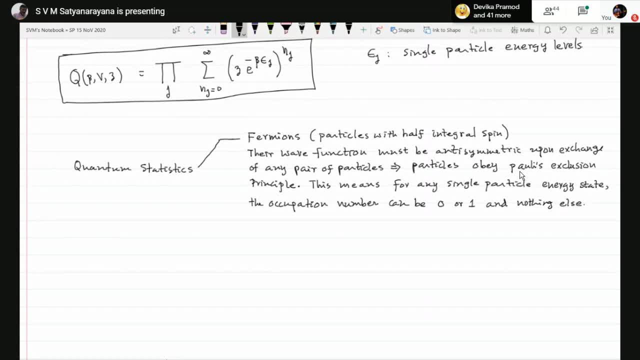 This is a very important statement because this is what happens, this is what distinguishing feature of Fermi analysis, So which implies that I can write down the grand partition function for Fermi derived statistics. let me set it as a function of beta in time set. 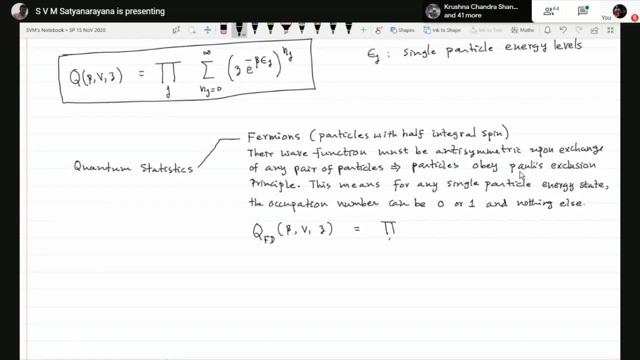 as rod of power k. rod of power j. Now this n? j for every epsilon j, this n? j can be equal to 0 or 1.. So that means it is empty or it is occupied with one part of epsilon. So 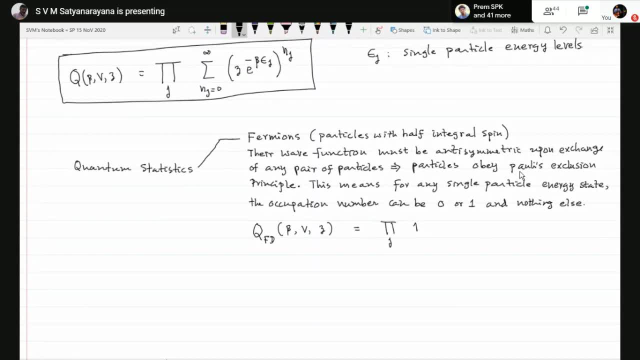 that tells you: if n j is equal to 0, I have 1,. if n j is equal to 1, I have z into e to the minus 1.. So this is the grand canonical partition function for Fermi analysis. we have Fermi. 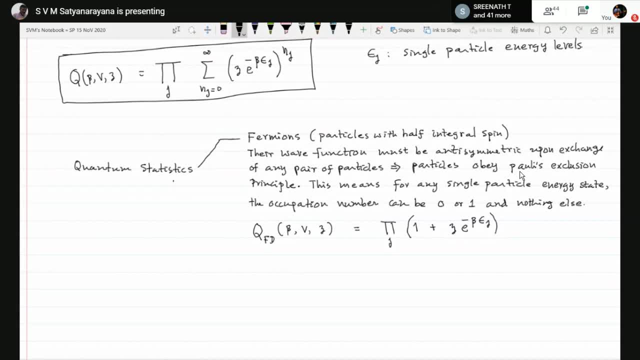 derived. Now, on the other hand, you have bosons, particles whose spins are integrals, particles with the integral spin, and where the wave function must be symmetry, must be on the spin spin of the wave. So there is no restriction because of the symmetric nature of the exchange. there is 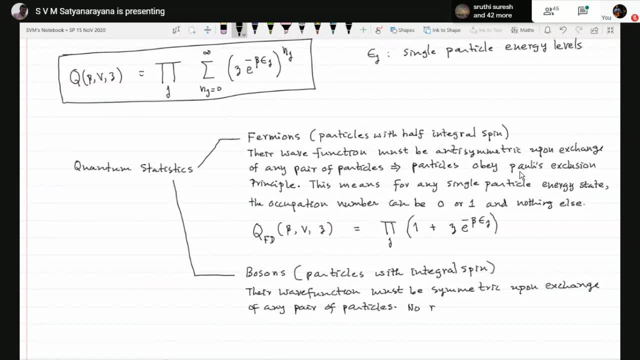 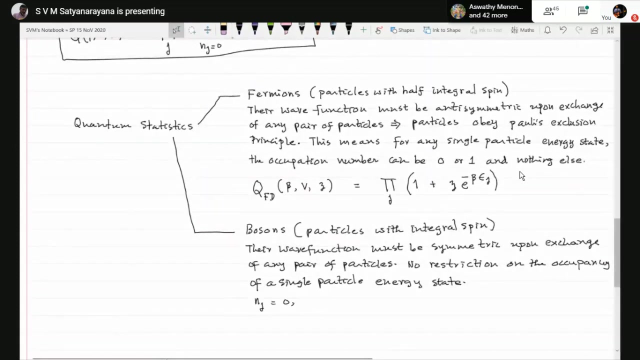 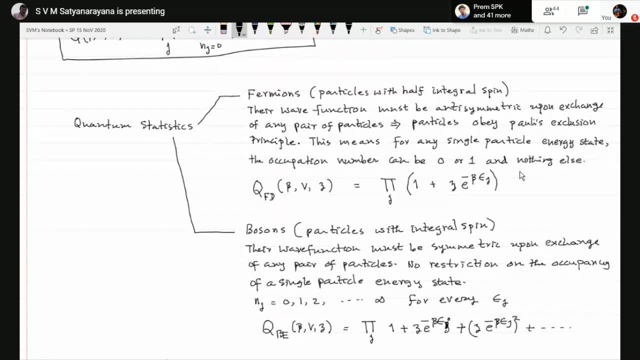 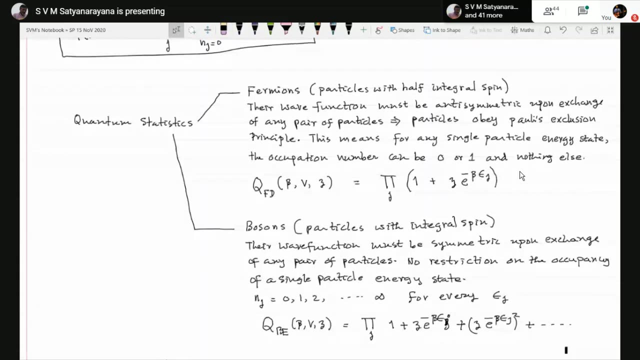 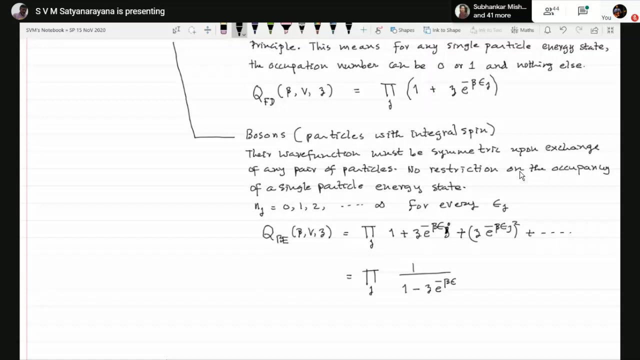 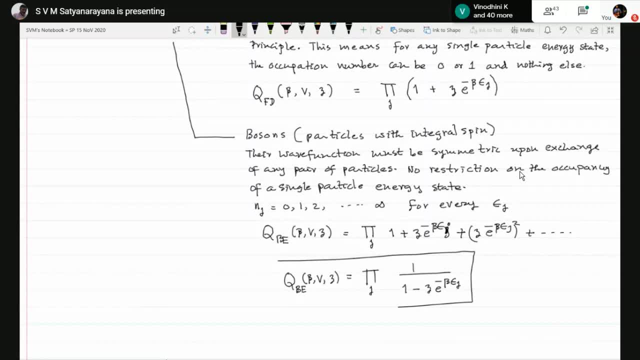 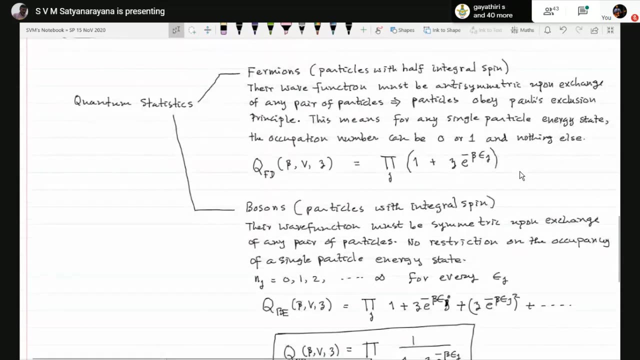 and so these are the statistics that you, in fact the articles. we get divided into these 2 categories. there is a relation. this relation relation between a spin of the particle, spin of the constituent constituent factor and statistics- Okay goes by the name spin statistics- spin statistics connection. 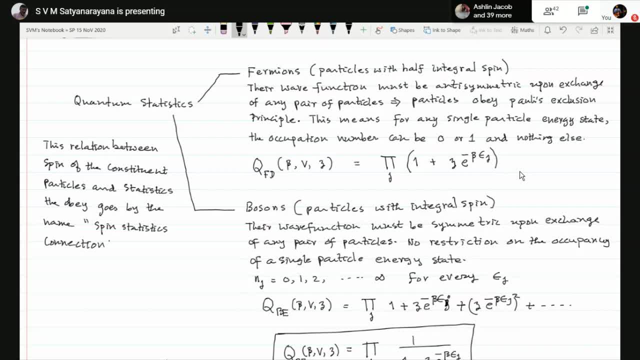 Okay, Initially this was supposed to have been given by Cowley, but this can be proved. this is the выставка. This is the. this is the statement. This is the. this is the statement. So over here, a family name. 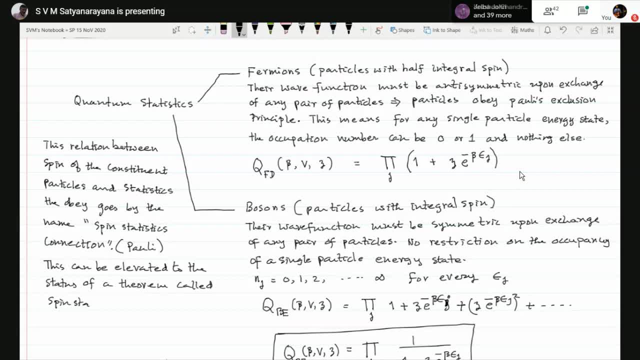 So this is a family name. Now let me, Let me show you, I want to show you a couple of examples. So say, we use a few terms, So then let me just show you. It's a kind of a technical term. 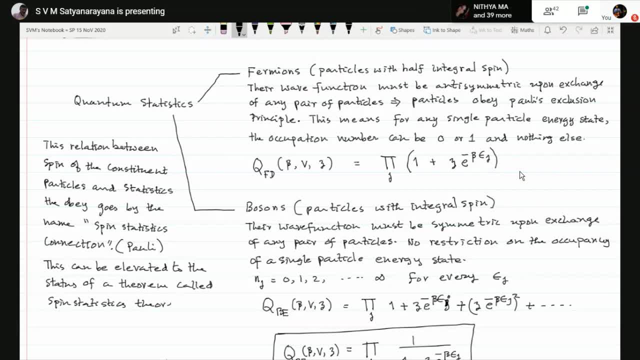 It's a funny term, It's a little bit more complex. for example, You know what I'm saying. Yeah, This is this is the. This is the, this is the term- can be proved using the tools of quantum field. 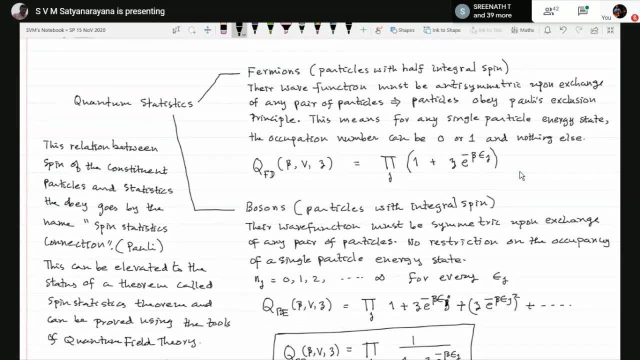 I just wanted to make this remark so that you can keep it in mind. if you study quantum field theory, You can keep this in mind and search correctly, But we are not going to look at it as a spin statistics theorem. I want you to understand. 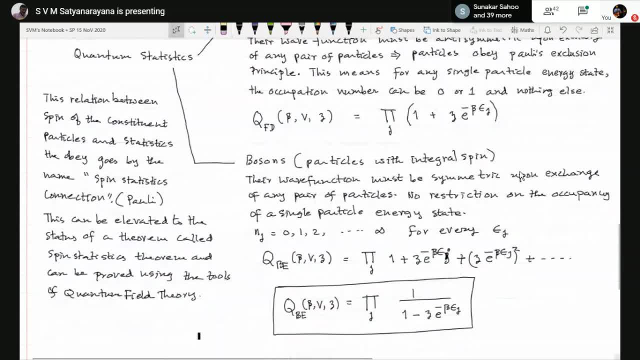 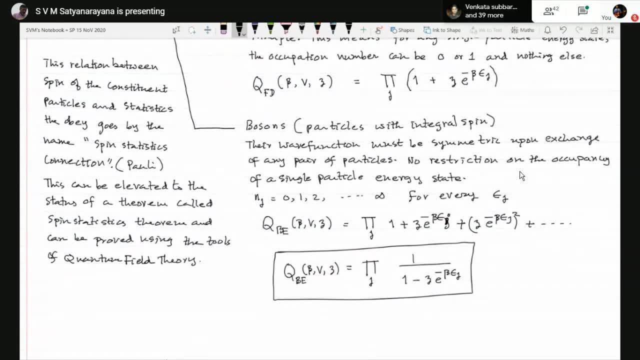 that there is a connection between the spin of the particles and the statistics, and that connection is what I have made here: the grand partition function. So we are going to look at the different particles, whether they are fermions or bosons, and the entire physics of the systems is also different. 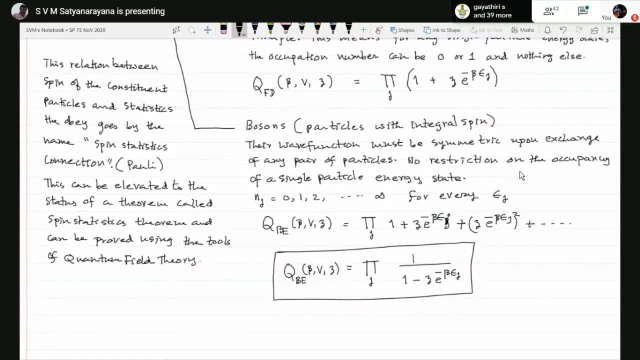 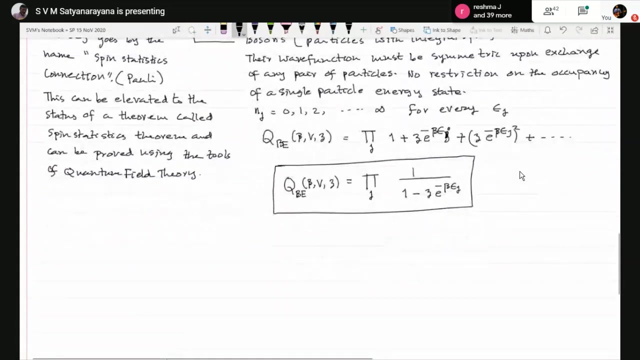 But notice that this is all because of nature of overlap of the wave. functions is different based on their spins. So once we have this grand partition functions, now you can ask, you can try many things. For example, first let us look at the single particle energy sphere. single particle energy. 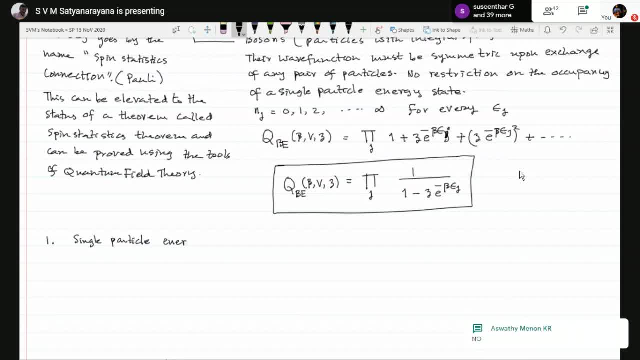 sphere. Okay, So let us look at the single particle energy sphere and how you can analyze thisEarea and then find out the other particulars. This is all working well. First this. So this you can obtain by asking what is the average number of pipe. So for that we 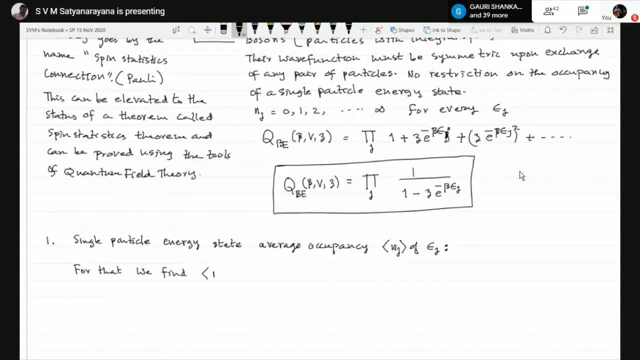 can find average number and average number. and this we can find because we know, once we have grand partition function, what the average number is. So we know that average number of particles obtained from the grand partition function by taking the average number of pipe. So let us look at Fermi-Dirac statistics, FD statistics. In the case of FD statistics, 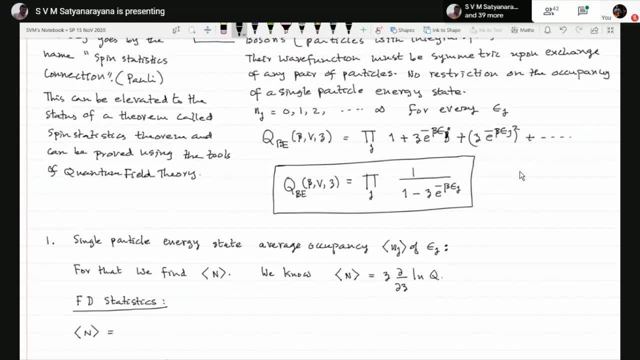 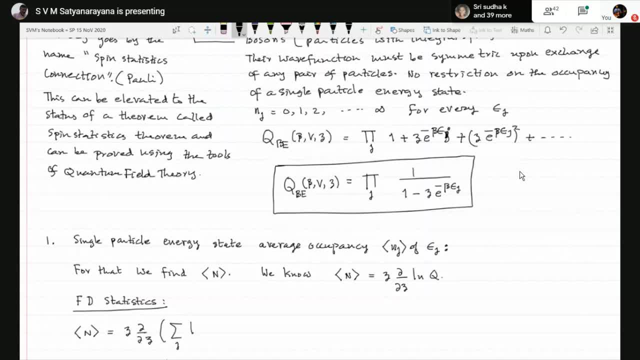 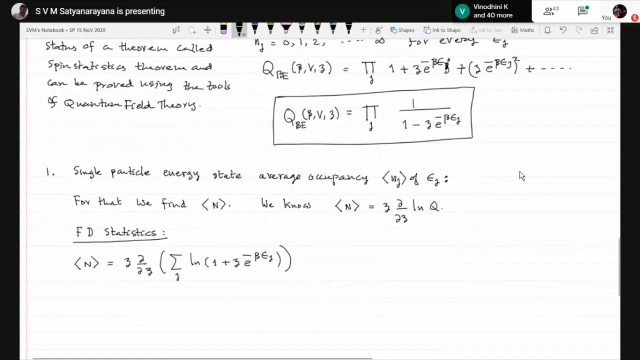 is sum over j logarithm 1 plus z e to the minus eta epsilon. So that is my estimate and you know I can. I take this since by some of a 1, by 1 plus said excellent a and the derivative of this term. 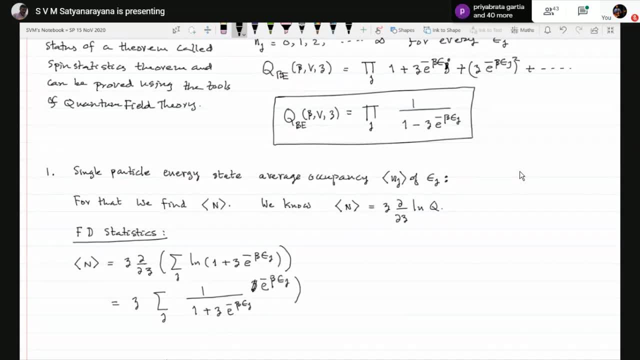 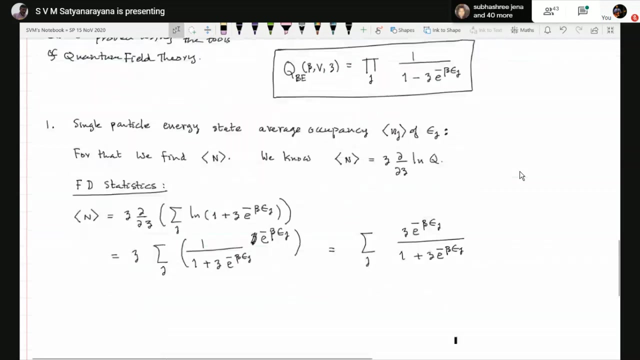 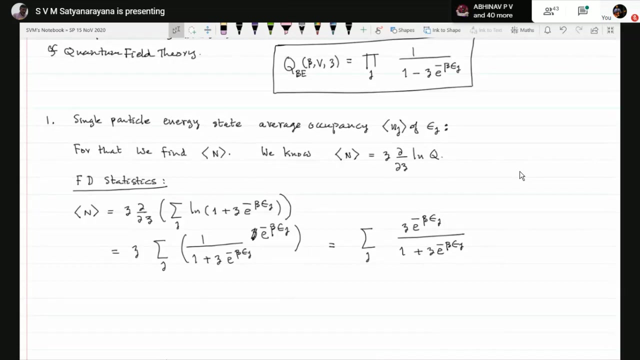 said during, e to the minus beta x. so this can be written as sum over J Z into e to the minus beta epsilon, a divided by 1 plus Z into e to the minus beta epsilon. so it is sometimes useful to write it in the following fashion: so we take this: 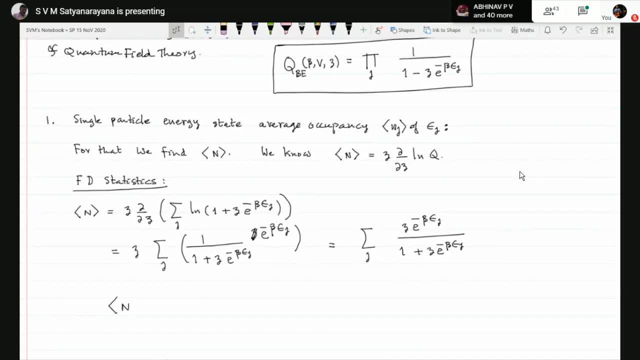 numerator to the denominator, and then write this n as sum over a, divide this as Z to the minus 1 into epsilon a, so which I could have written it as sum over J average number of particles in each of. okay, so if I, if I write it, 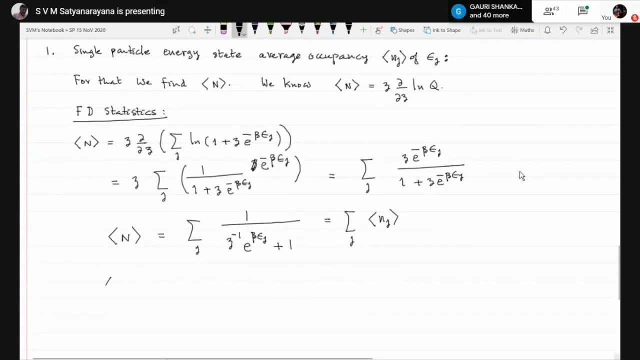 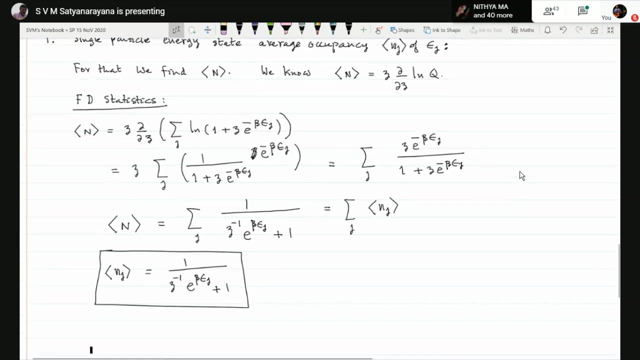 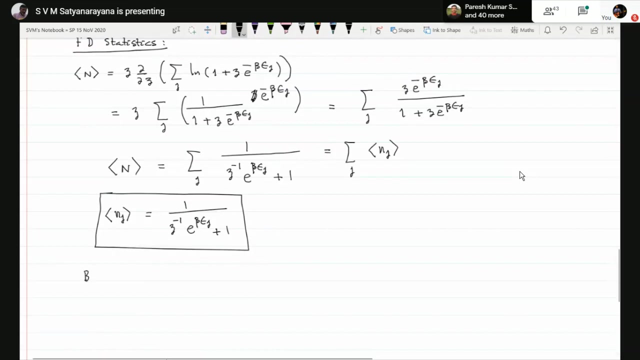 like that. then I have the average occupancy of a single particle energy state n a, which is given by 1, divided by Z to the minus 1. so this is an expression oraverage occupancy of permeability. Now let us look at the case of quotient state statistics. Let us say I have e e state If 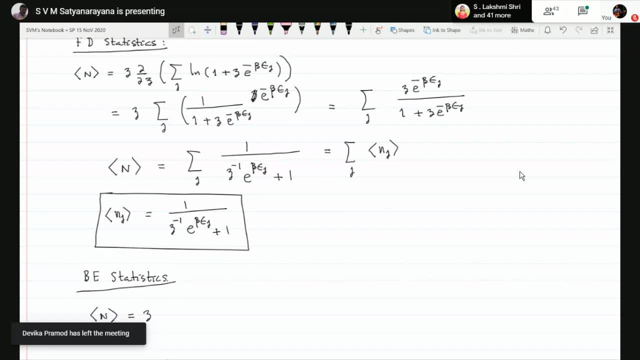 you have b and your average n is equal to z, 4 by j z of. so you have a minus sign and I have sum over i logarithm of 1 minus third j j minus theta j, because that is 1 by 1 minus j j by minus theta j. 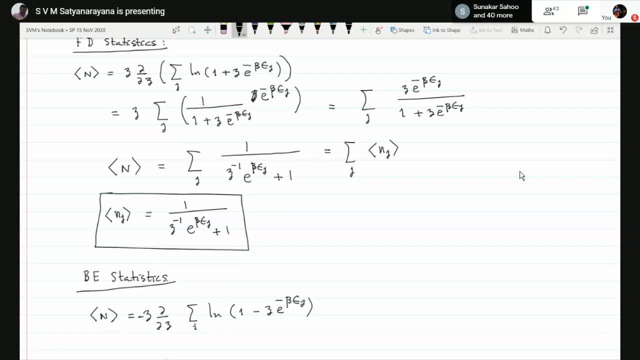 When I take logarithm I get a minus sign out. So that is what. So this also you have. you can do a similar thing. Then you will have sum over j z e to the minus theta epsilon j, divided by 1 minus z e to the minus theta epsilon j. 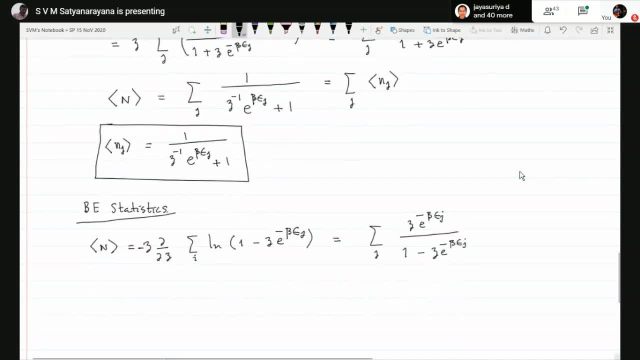 So once again I can take this numerator to the denominator and then write this n as this number and sum over j, 1 by z inverse e to the power big log theta j minus 1.. If I write it as sum over j, n, j. 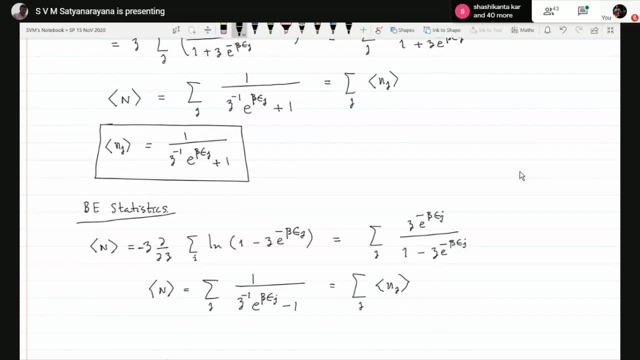 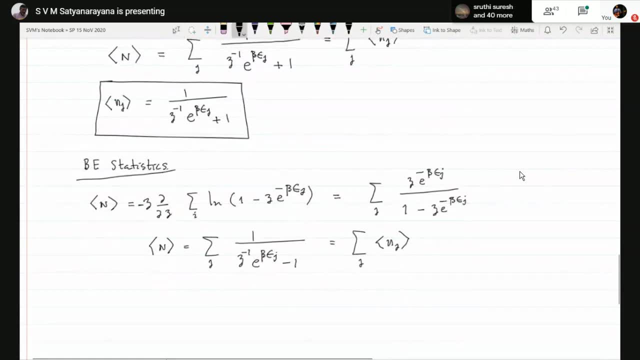 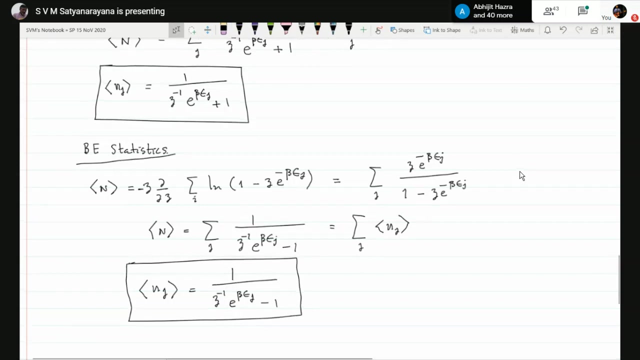 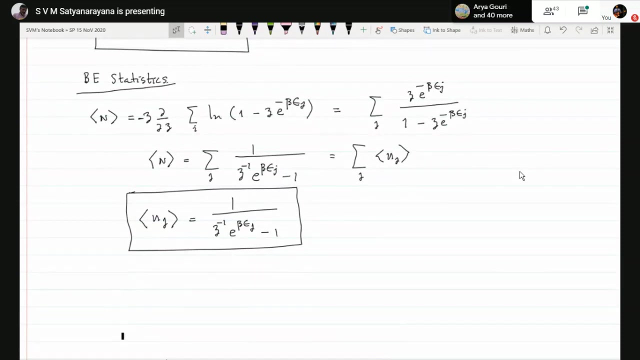 Okay. Okay, Then you have a, So I have a minus sign. So I have a minus sign Okay for the occupancy presently. but a is equal to 1 by the universe is the power of the universe. Now there is also interesting. it will be. 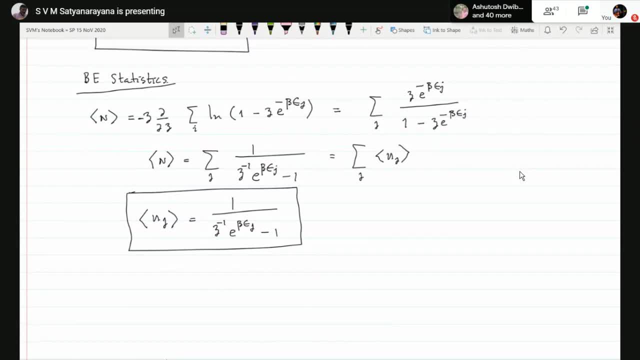 interesting to see what happens if these are classical particles. So classical particles, that means classical particles. they obey what we already know as Maxwell Goldman's statistics. So we will try to look at Maxwell Goldman's statistics in the same occupation number, representation. Now, what happens is so, if you have classical particles, that 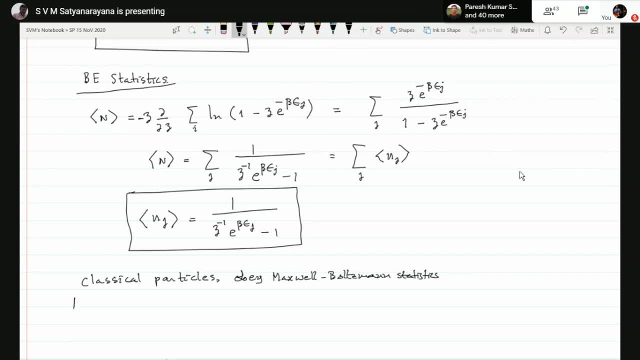 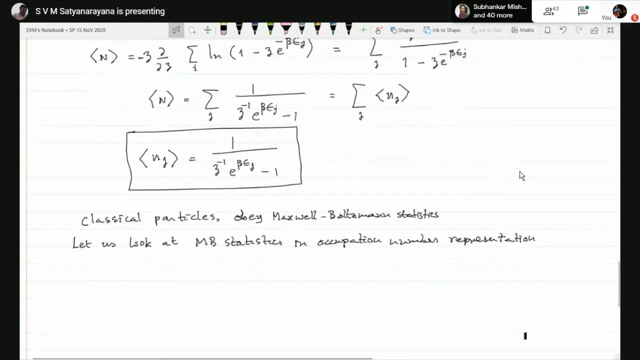 means: let us deal And let us look at Mb statistics in this occupation, member representation, expression of that is for a given, for a given mode of this n? j, there are factorial n divided. 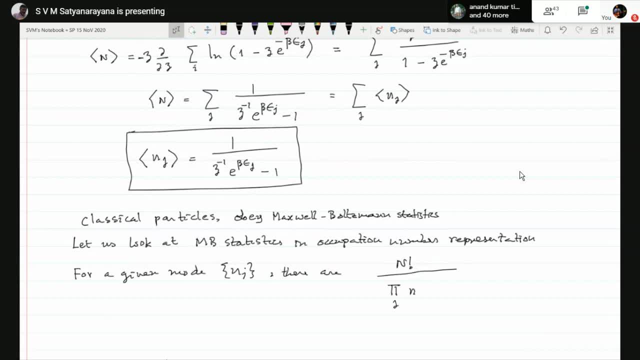 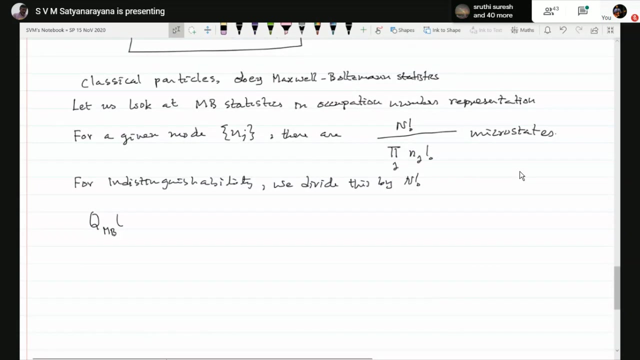 by product over j factorial n, j microstates. ok, So these many microstates are there and and for for indistinguishability, we divide this by factorial j. So if you do this, then what happens? if you have a a true Maxwell Boltzmann of beta unit n right is going to be equal to somehow where music. 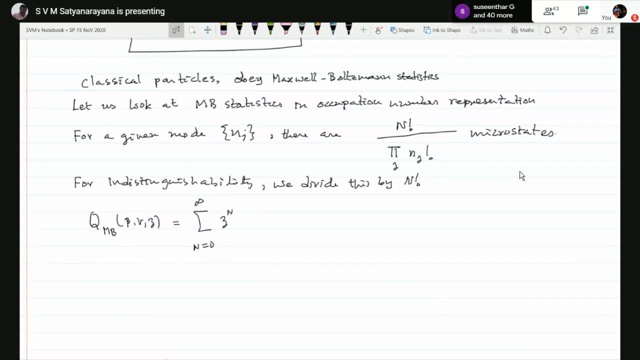 is pure. So if you do this, then what happens? if you have a true Maxwell Boltzmann of beta unit of here to the n and somehow, where we have this sum over b n j and the constraint, the sum over j n j equal to capital n. Now we have one by product over j n j equal to n. 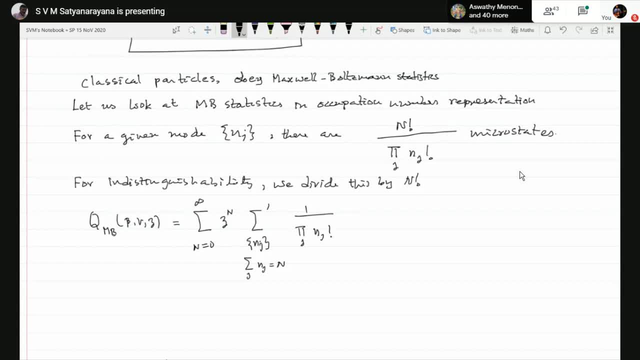 by factorial and this capital N factorial will be cancelling because we are dividing by capital N factorial into e to the minus beta, sum over j, epsilon j n. So if you use that result then you can write this as product over j and sum over N. j is 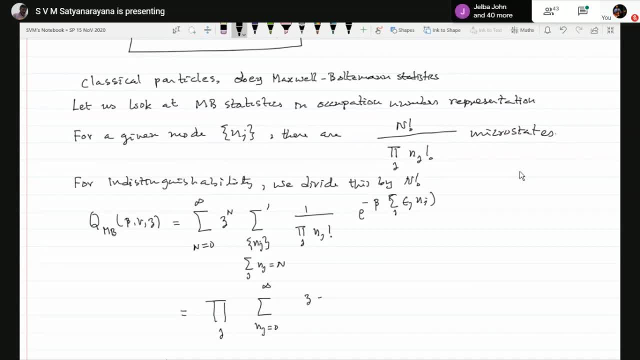 equal to 0 to infinity, that e to the minus beta, epsilon j to the power N j divided by factorial N j. this is what we will have, Because there is a product over N j sitting. for each of the term, you will write that: 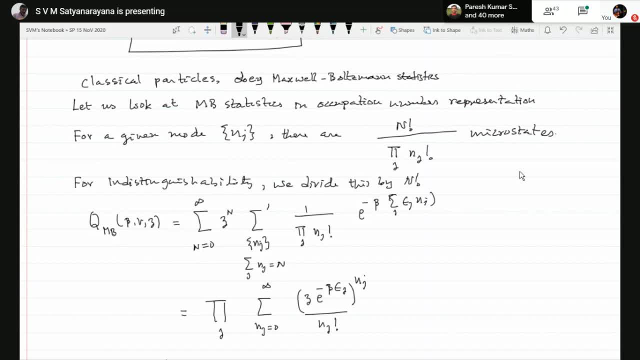 N, j factorial, and this is what we will have. But this summation is well known. so this is nothing, but you have product over j, exponential of that being e to the minus beta i. So this is E power, x is x. power N by N factorial N is equal to 0 to infinity. 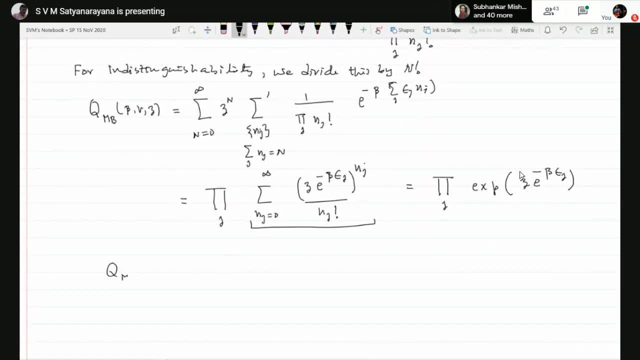 So the grand canonical partition function for Maxwell-Boltzmann statistics is beta v. z is equal to product over j in the partial unity levels, exponential of z, e to the minus, e to the epsilon. Okay, Thank you, Thank you. Thank you for your attention. 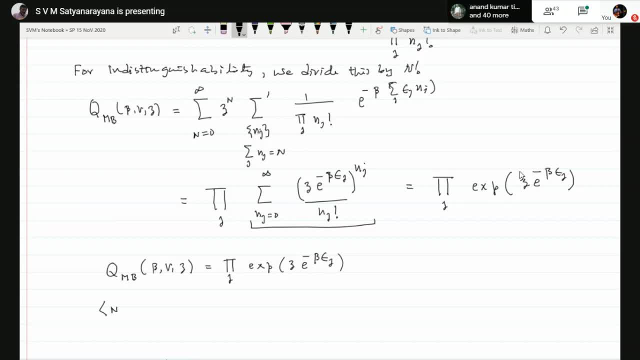 And suppose, if you are interested in finding out average number of particles again, is z equal to z, the product becomes sum and logarithm of this z into e to the minus beta logarithm exponential will cancel and you have. This simply gives you that this is sum over j. 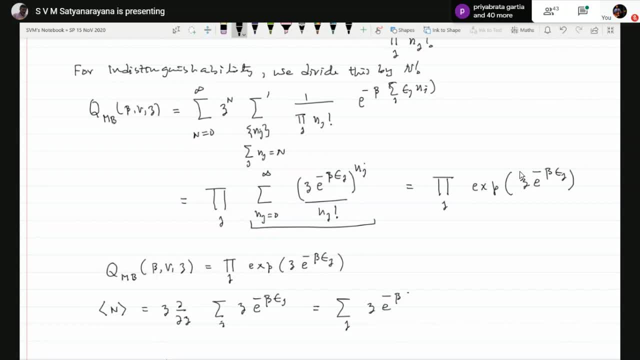 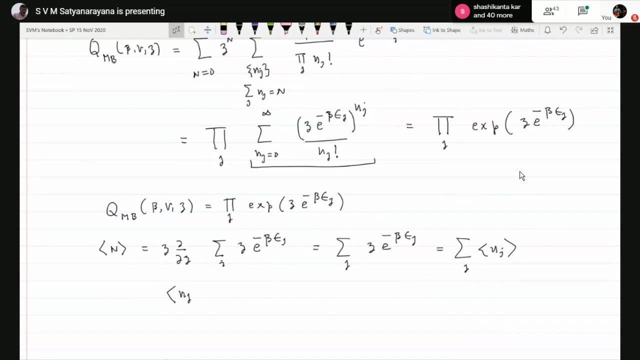 Thank you, Thank you. z e to the minus beta And if you are writing this as some of the n, j, so the average occupancy of a Maxwell-Bosnian under Maxwell-Bosnian statistics is simply z into e to the minus. 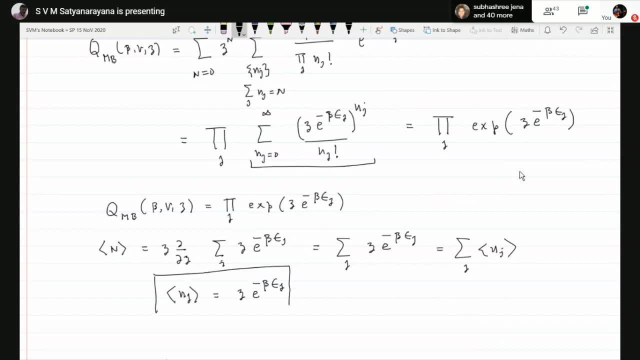 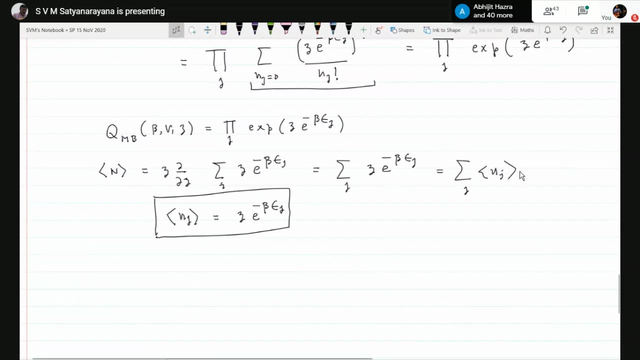 beta. So we have expressions for average occupancy of single particle energy levels in the case of three different statistics: Classical statistics, which is what is called Maxwell-Bosnian statistics, and quantum statistics, Fermi-Dirac statistics, and both. Now, looking at these expressions, it is suppose if I write this as z to the minus beta, then 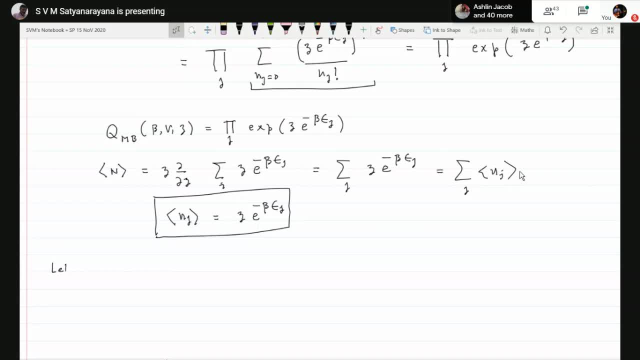 I can write this as z to the minus beta. So let the epsilon be a single particle energy, single particle energy of an energy state, And let average n epsilon be its average occupancy. Sir, in classical system isn't the particle distinct visible? 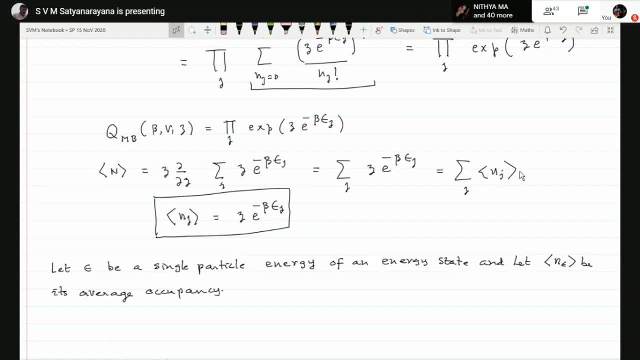 You can track every particle. Yeah, So in classical system we have there is some indistinguishability at the level of permutation of this particle, Just like what we discussed in the case of Gibbs paradox. So I am dividing this as the factorial n you take care of that kind of an indistinguishability. 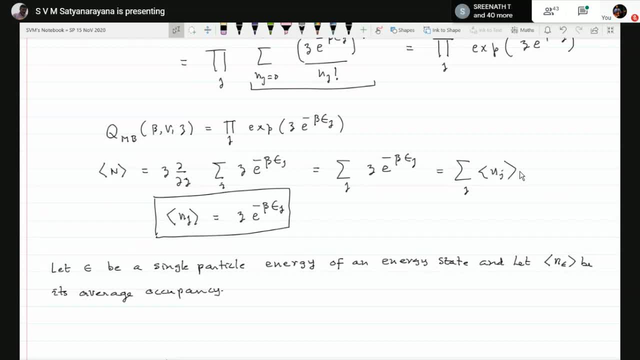 Okay, Whereas in quantum statistics actually there is no. they are identical. That means you do not have this kind of continuity. That is why I did not put any weight when I did quantum statistics. Okay, So this is what we are going to do. 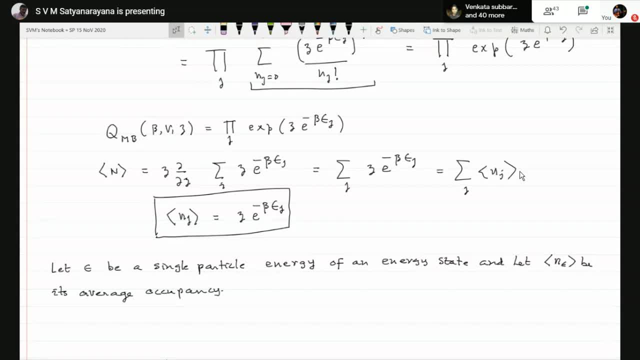 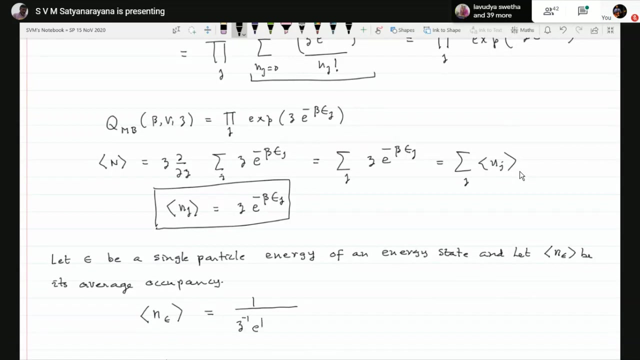 Okay, So this is what we are going to do. Okay, Anyway, we will. So this I am going to write as 1 by z to the minus, 1, into e to the beta, x, inverse, Okay, And I am going to call it as plus some a, okay, And I am going to say that this a is: 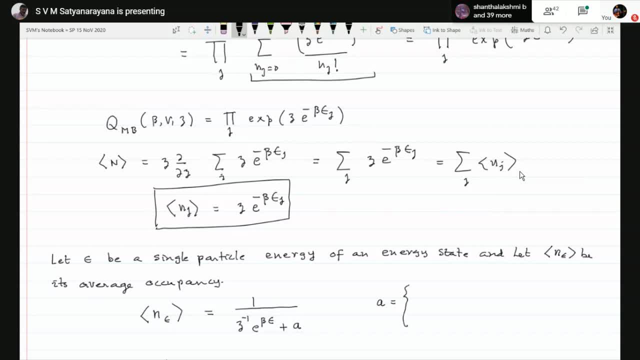 equal to plus 1 for Chudney-Dirac statistics and this is minus 1 for Bose-Einstein statistics- Okay, And it is 0 for Maxwell-Bugner statistics- Okay, It is easy to remember once. So this is a unified expression where there is a constant a that is changing other things. 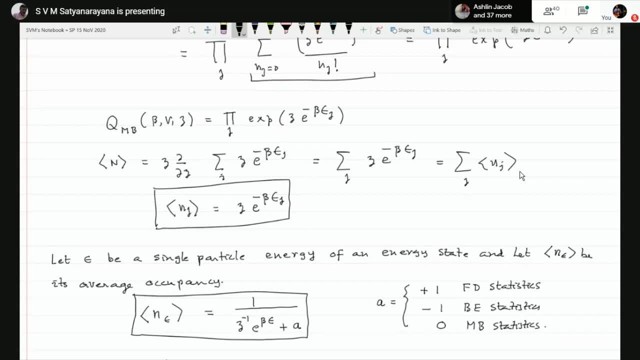 are all same. So for Chudney-Dirac statistics, a is plus 1 for Bose-Einstein statistics: Okay, So this is a constant a that is changing. other things are all same. So for Chudney-Dirac statistics, a is plus 1 for Bose-Einstein statistics. 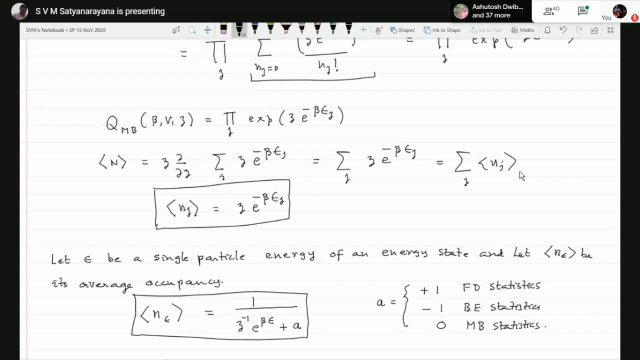 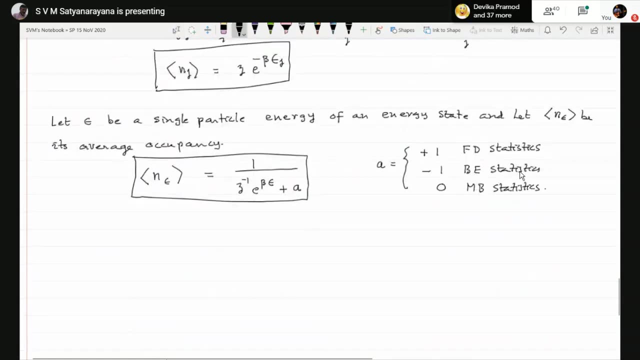 Okay, So this is a, So this is average occupancy. Now, the average occupancy also has an important, For example: consider, let us say, consider- the error. What is error? What is the error? What is the error? 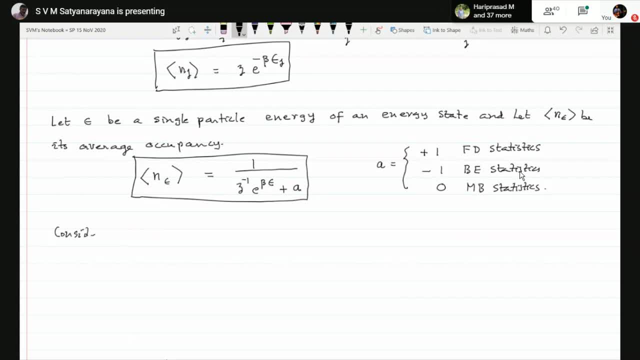 What is the error? I will consider the case of case of FD statistics. ok, So if you consider the case of FD statistics, you know this average of frequency given by 1, by z inverse plus e, to the beta epsilon plus 1. ok, Now your single particle level. let us say this is the energy level. there are 2 possible. 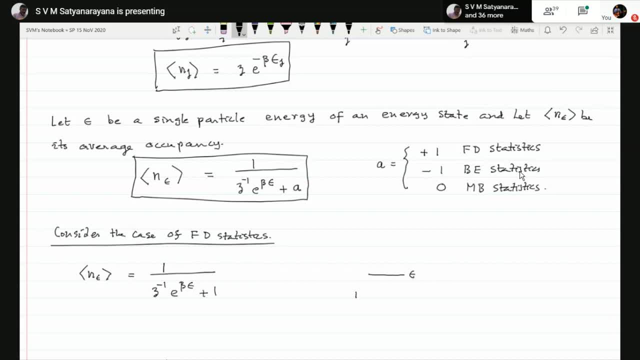 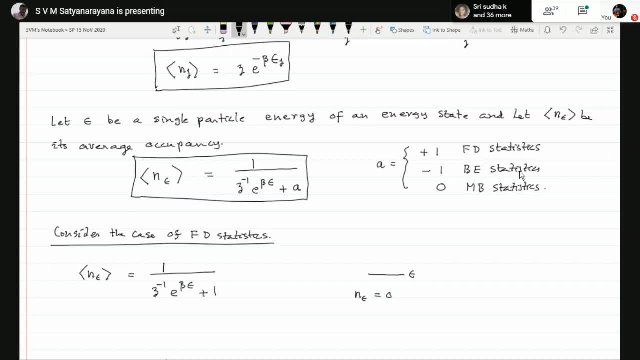 of the particle. So this is the energy level of the particle. So this is the energy level of the particle. ok, So if you are, if you have n epsilon to be 0, then the energy of that so energy is 0. or you can have a possibility that n epsilon is equal to 1, in which case 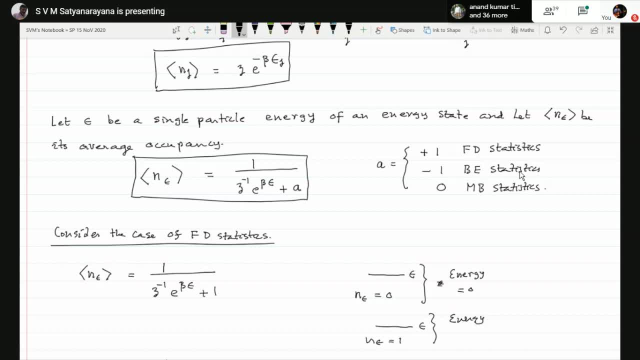 the energy is energy, that is Theются. ok, So that means I have. it is like I have two microstates. ok, So I have two microstates of A is 0 and epsilon. it is like two level system, correct, it is like two level system. 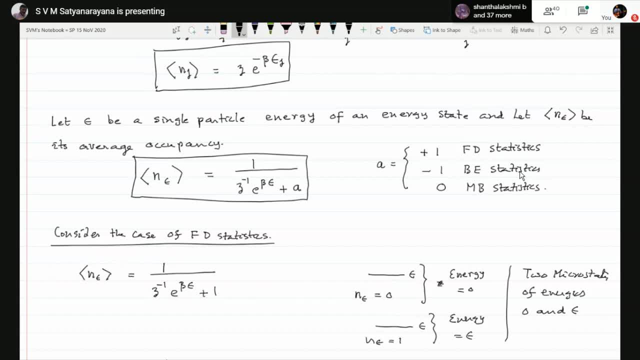 Now suppose, if I am asking you a question that what is the, what is the, what is the grand partition function for this? So let me call that as some Q. So the grand partition function for this is: it is like z into e to the minus beta epsilon. this is your Gibbs factor, this. 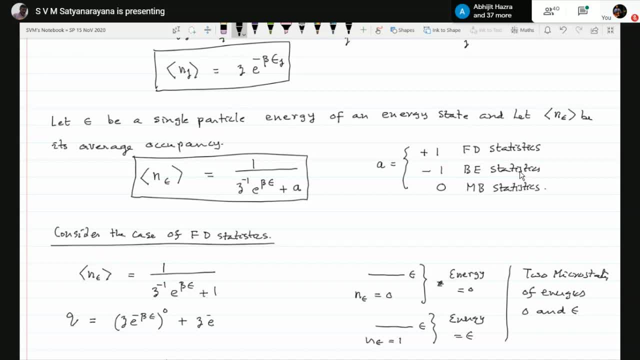 to the power 0.. power 0 plus z into e to the minus beta epsilon is to the power 1.. So that means that is equal to 1 plus z into e to the minus beta epsilon. This is your grand partition. 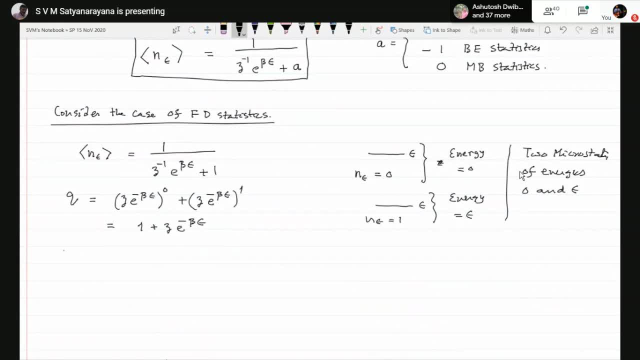 Now you can ask a question that: what is the probability that the energy level is occupied? What is the probability that the energy level is occupied? What is the probability that the energy level is occupied? That means the probability that your n epsilon is equal to 1. That means it is occupied. That is equal to z into e, to. 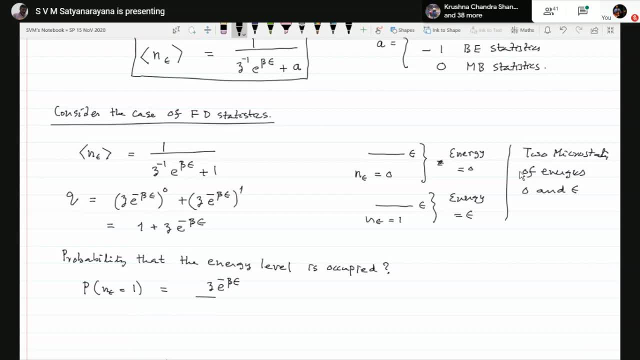 the minus beta epsilon. This is the Gibbs factor divided by q, So which is equal to z into e to the minus beta epsilon, divided by 1 plus z into e to the minus beta epsilon. So I take this numerator to denominator and I have z inverse e to the beta epsilon. 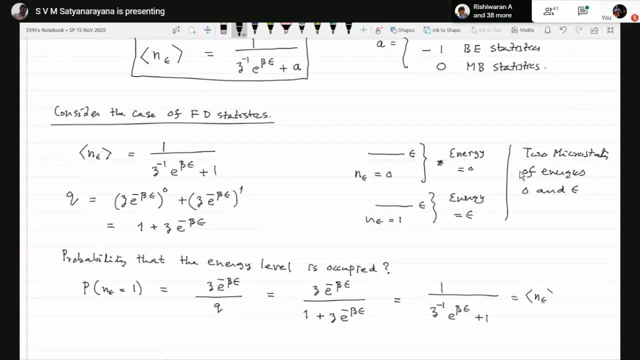 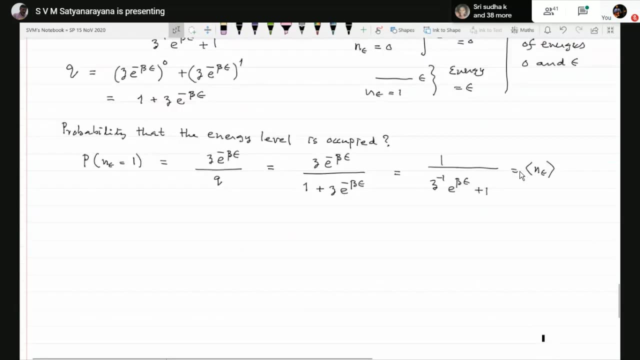 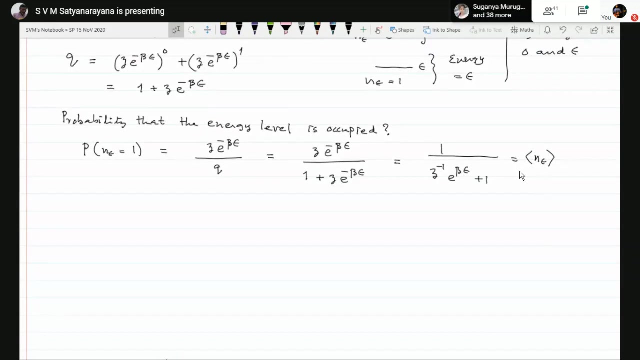 which is same as average occupancy. So that means the average occupancy is same as the probability of the occupancy. ok, So the probability of the occupancy is same as that of the energy, energy of the occupancy. ok, So this is something which you have probably. 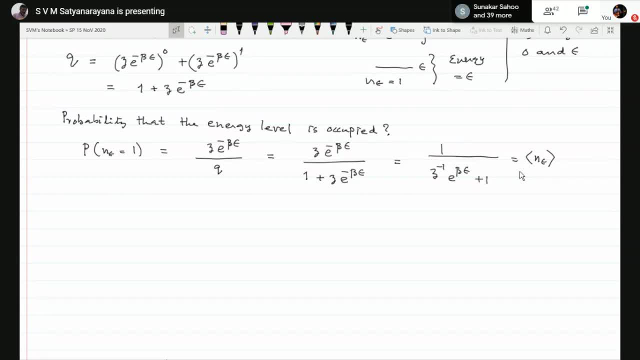 seen in when you do electrons in metals in solid state physics, that we consider this probability and you say that at t equal to 0, the probability is 1 up to thermal energy and 0 beyond thermal energy. So this is the expression which you use to find out the probability. 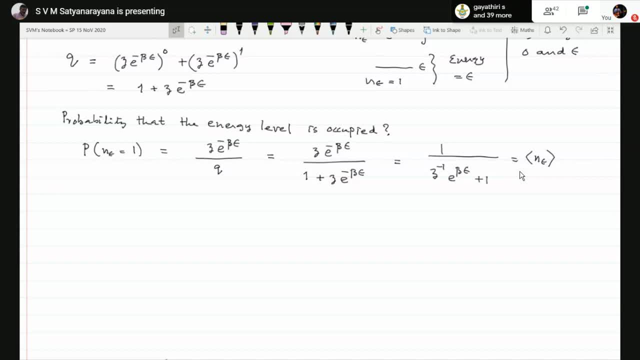 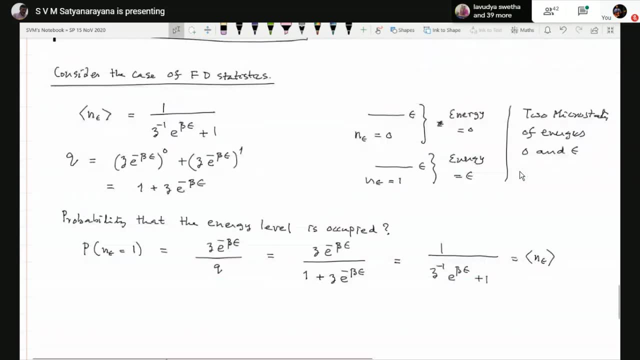 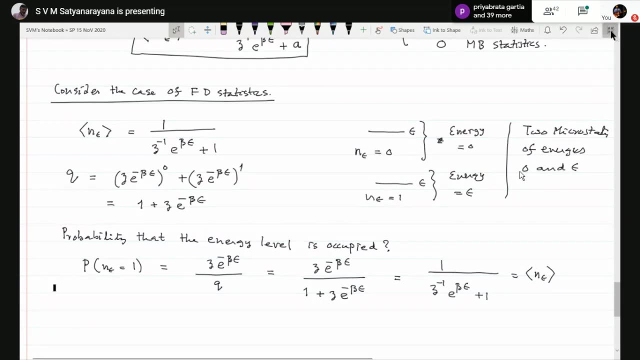 various properties of electrons in metals. So this is the use of average occupancy. So remember that we have been continuously talking about single particle energy levels and that is possible because we are, we are able to, we are able to get it to do that, because 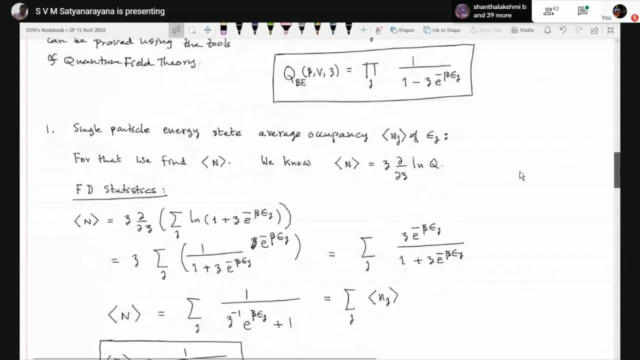 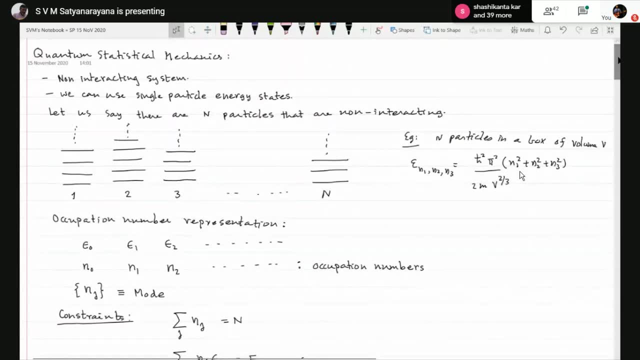 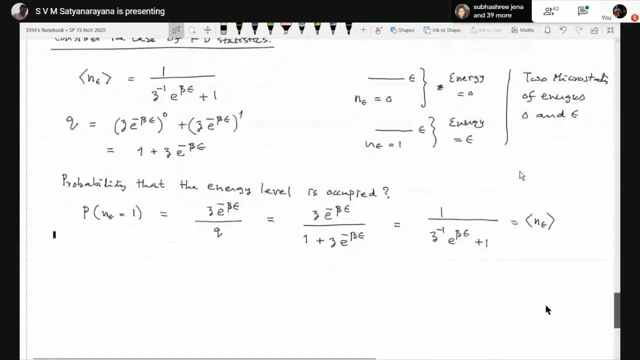 we are using non-integral energy. So this is the expression which you see in the slide. So this is the expression which you see in the slide. So this is the expression which: So this is the expression for average occupancy of each one. Now look at this expression. 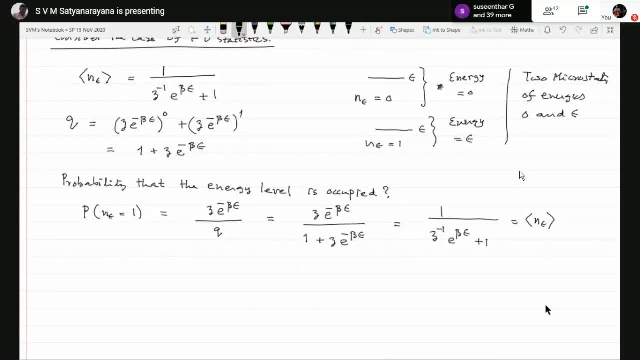 even though it is buried like this z. what is our z? Our z is namely the fugacity which is given by e to the power b times. ok, this is fugacity and u is here 10 times. ok. So if you are writing, if you are explicitly writing that then the probability of n epsilon at 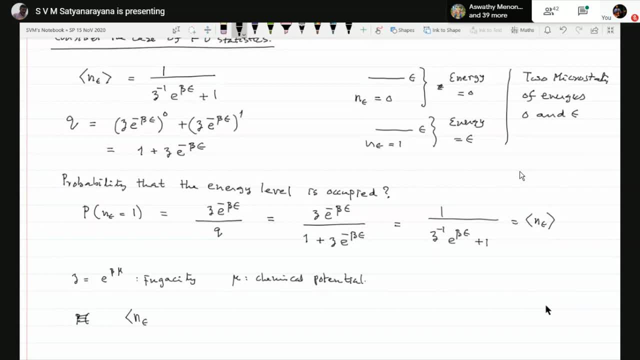 let me put it like this: So this is your n epsilon average n epsilon. in terms of this one, you can write it as e to the power z inverse. z inverse is e to the minus beta mu, So I have e to the power beta. 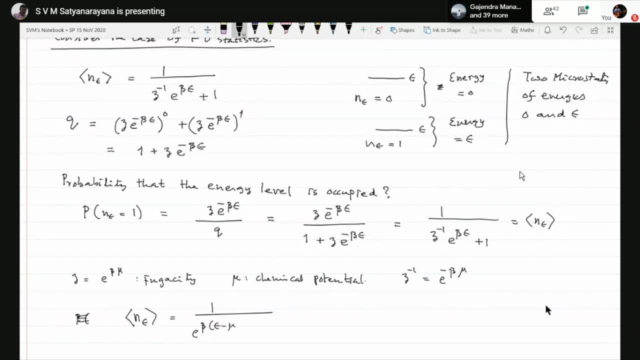 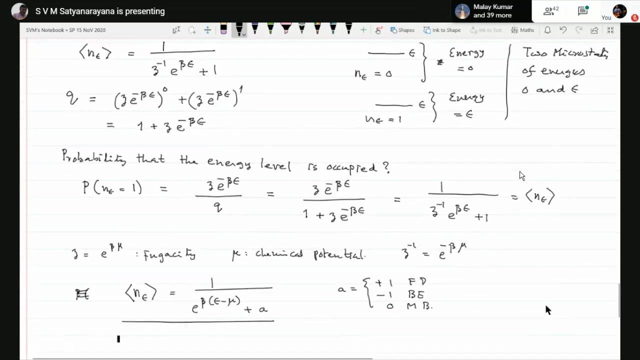 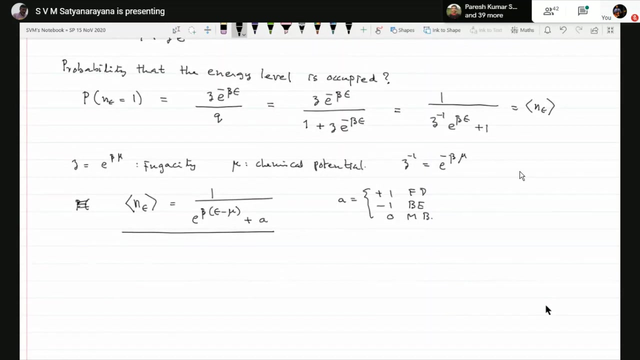 into epsilon minus mu, plus a and a is equal to plus 1- correct me- And minus 1.. So b 0, 10.. So this is what is in terms of Now, supposing. if you are interested in asked in what are the possible values, Suppose, let us denote beta times. 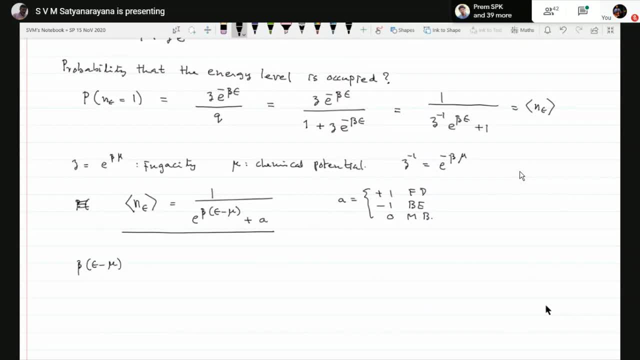 epsilon. So 2 beta 3 to the power n epsilon, beta to the power, beta into epsilon. So what minus mu? theta times epsilon minus mu? let us call it as some x, And then your average number of epsilon becomes 1 by e to the x plus a. ok, 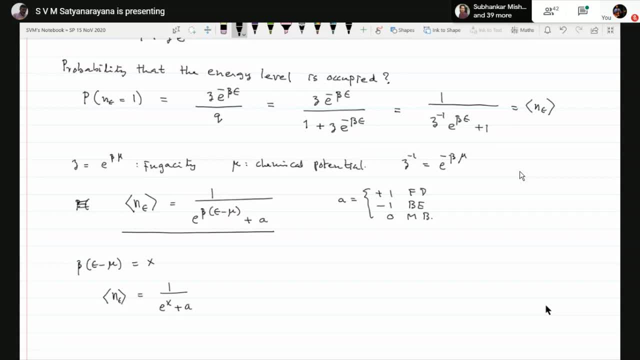 So now, supposing, if I want to ask, what is the value that your x can take? ok, So, for example, let us look at, let us look at Fermi-Bedard statistics, FB, FB statistics, ok, And if you, 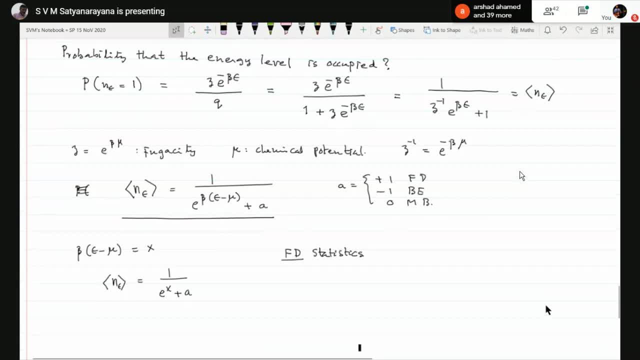 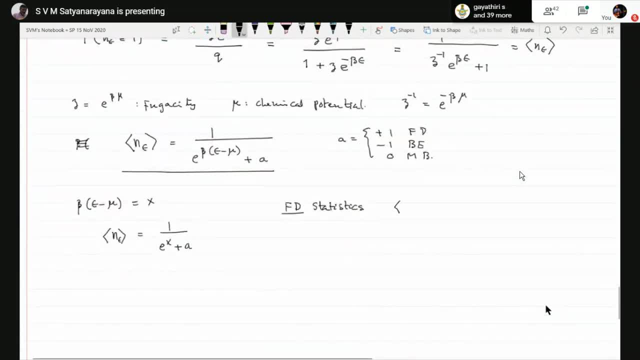 So if these statistics you have, average number is equal to 1 by e to the x plus 1.. Now, at x equal to 0, your average n epsilon is half, and as x tends to infinity, then average number of epsilon is equal to 0. And as x tends to minus infinity, then average number of particles. 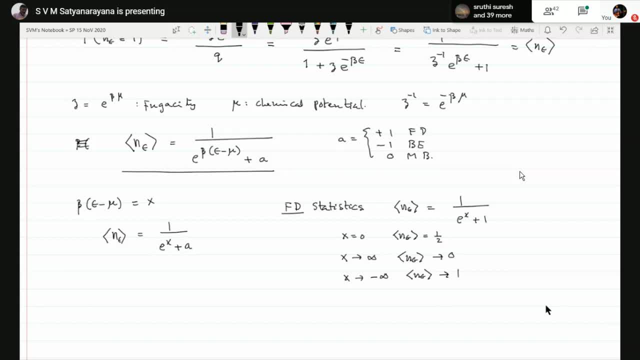 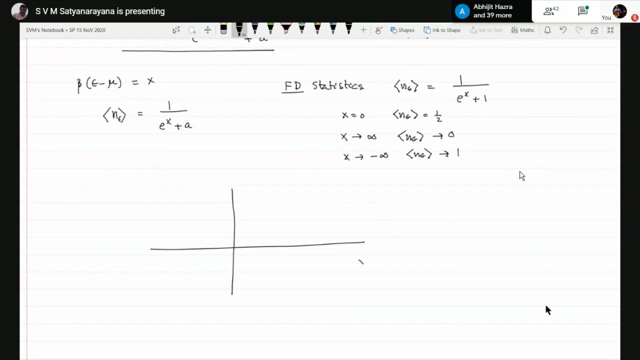 will go to 1.. So this is the behavior of this function. So if you are trying to plot this function Of x, let us say: let us look at x versus this average number, So you can see. let us say: 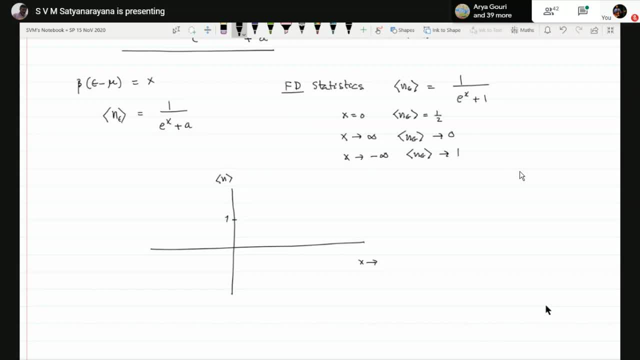 this is, let us say, 1, and this is half. So you can see that it goes to 0 and then it goes to 1.. And it will go through this half. it may not go so fast to 1, but this is how your Fermi. 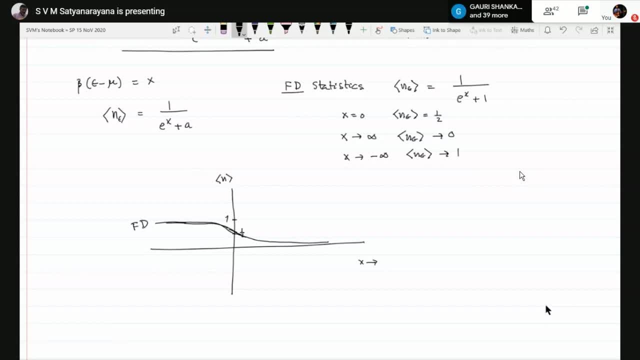 did that. ok, Now let us look at Bose-Einstein statistics. Bose-Einstein statistics: your average number in terms of n epsilon is equal to 0. So this is the average number in terms of this. x is 1 by e to the x. If x equal to. 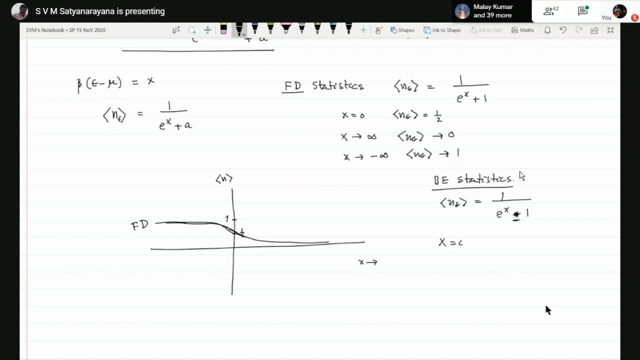 0. sorry, this is minus. So x equal to 0 implies this n epsilon goes to infinity. Now if x is negative, Then average n epsilon is also negative. but this is unphysical. This is unphysical because average number of particles occupying can be 0 or positive. it cannot be negative. 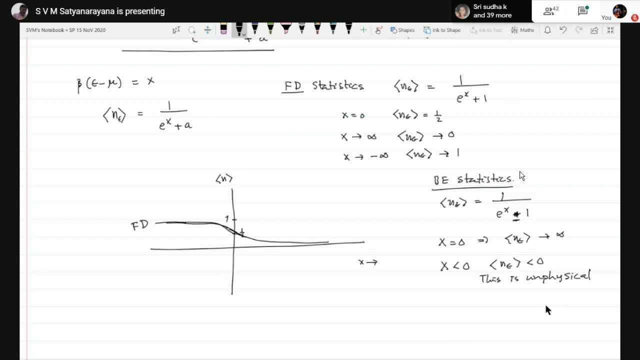 So this is unphysical. That means x less than 0 is not allowed. So x less than 0 is not allowed. So x less than 0 is unphysical. Now what happens if x goes to infinity, as x goes to? 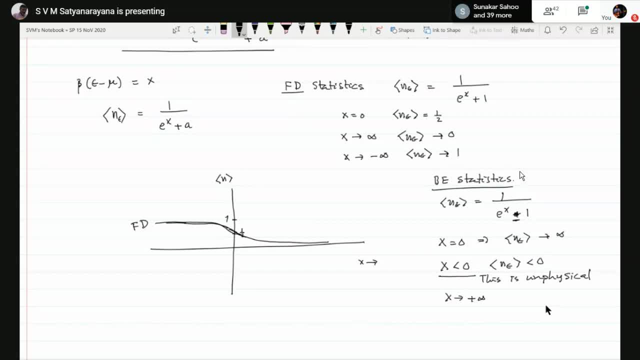 plus infinity and x goes to plus infinity. that means with n, epsilon goes to 0. So that means the range of this x is only between 0, less than, or x and less than 0. Whereas in this particular case the range of x is minus infinity, less than x, less than 0. So 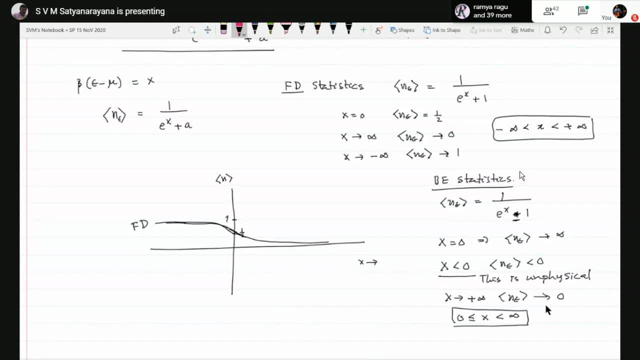 if you are interested in looking at how this looks like on the same plane, you can go to the same graph, So you can see that it go to infinity as x goes to 0, and then at some point it will merge with this one, So this will be what you call as cosine tensor. 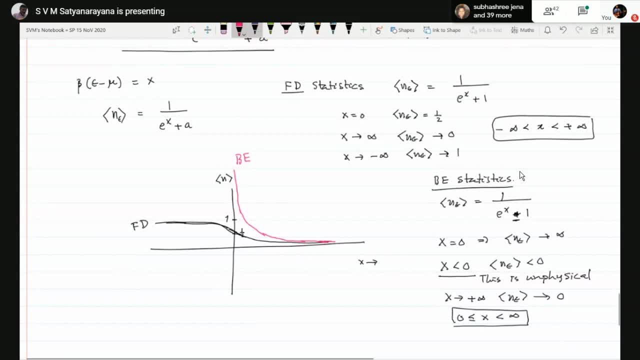 And what is your Maxwell Bozeman statistics? Maxwell Bozeman statistics is a very simple thing. So, Maxwell Bozeman statistics, that corresponds to a equal to 0.. So your average n epsilon is simply z into. ok, it is simply e to the minus x. So e to the minus x is something. 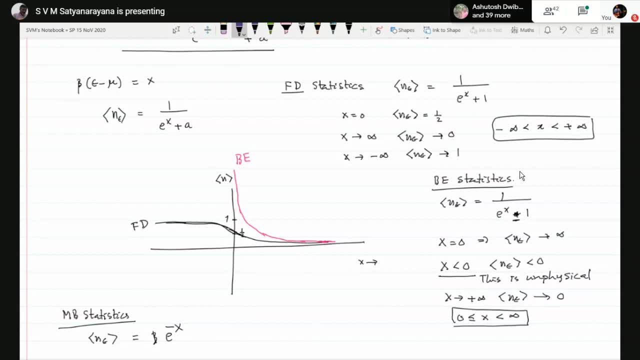 which you can draw, for example, So you can see it will come to 0. So you can see it will come to 1 here and then it is exponentially decaying. So this is your MD, So MD statistics also do not have. So MD statistics also has a relation. 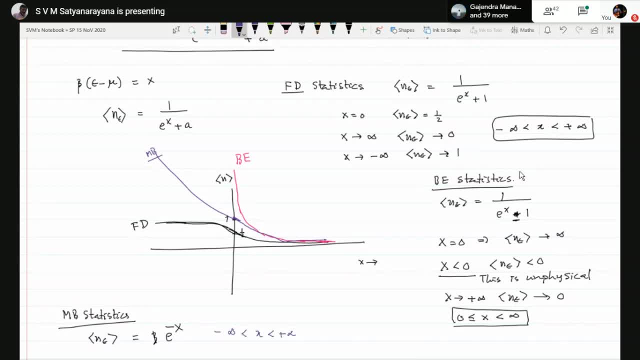 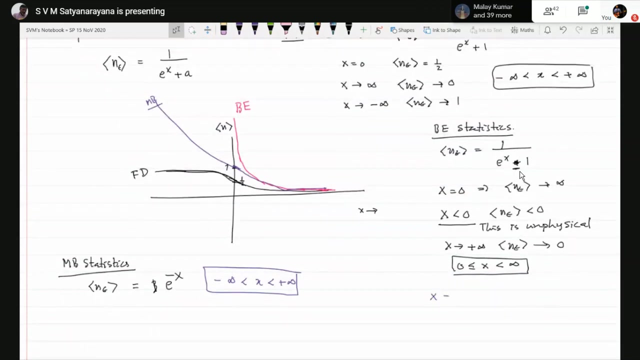 that minus infinity, less than x, less than infinity. ok, So if you see, the this Bozeman statistics has got a restriction in terms of the range of this x, and this restriction is it has a very important physical, physical relevance. ok, So if you look at x, if you look at x carefully, x is nothing but epsilon minus mu by a to. 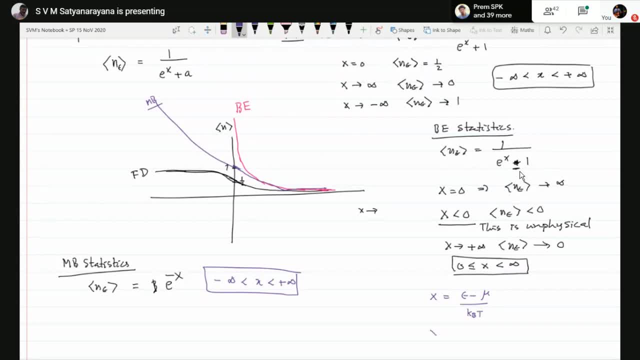 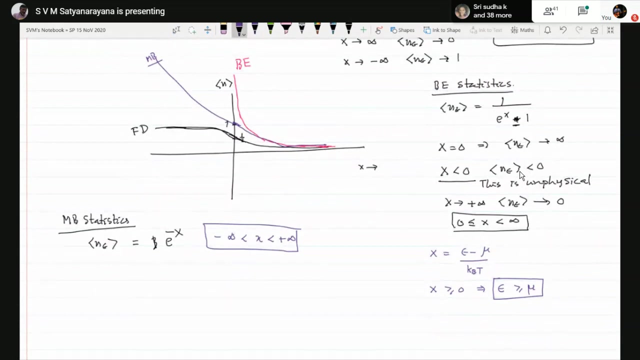 the minus x. So x has to be greater than or equal to 0.. This implies your epsilon has to be greater than or equal to mu. ok Epsilon has to be greater than or equal to mu. What does that mean? That means, if you are, let us say that. if you have, let us say that. if 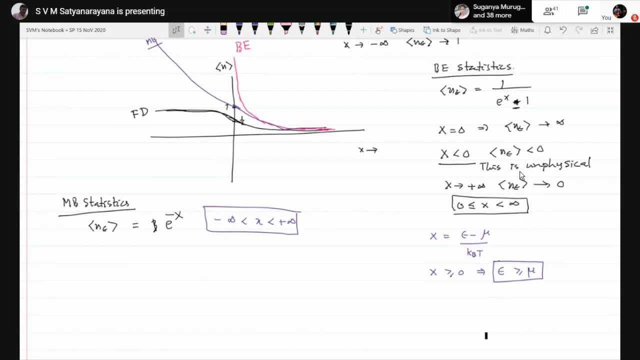 you have. so if you have ground state, for example, the ground state is 0, ok, So if ground state is 0, ground state is 0, let us say, epsilon is equal to 0. So if you have ground state is 0, ground state is 0. So if ground state is 0, ground state is 0. So 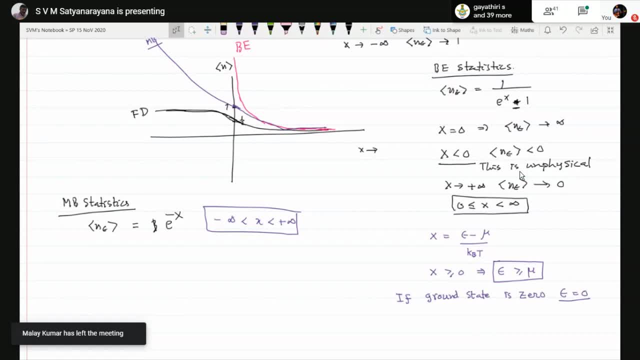 if epsilon is equal to 0, then it has to be equal to mu. that that implies your mu is also equal to 0. ok, What does that mean? If mu is equal to 0, that means there is no cost in adding more particles to that energy state. 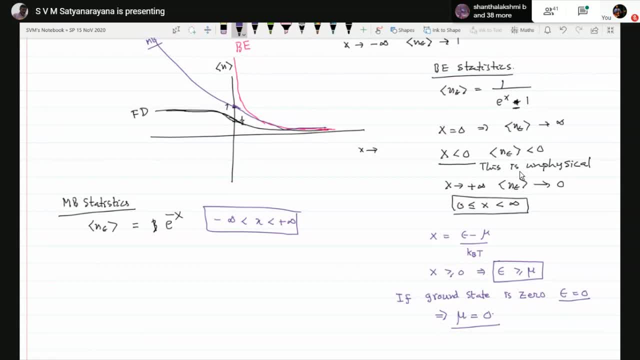 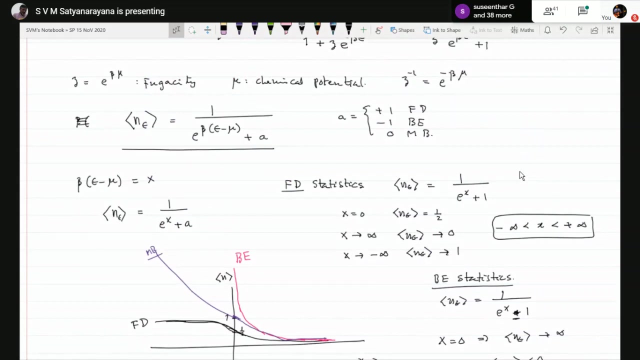 So this has very important implication for both arms. Okay, so we will discuss that when we are discussing both systems, but just notice that the minus sign that is sitting there, that a is equal to minus 1- makes a huge difference in terms of bosons and fermions. 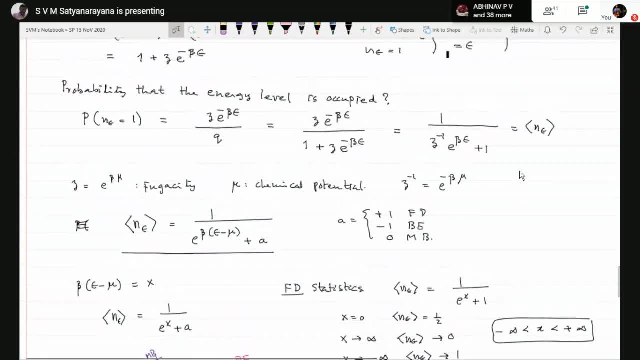 So that plus sign, minus sign is what makes aunuz lettere. So in this volume system there one should have zero free space threshold. if we have space perímetros, This would be a limit of this volume systemK that we will be using in theそ. therefore, this is 0.. 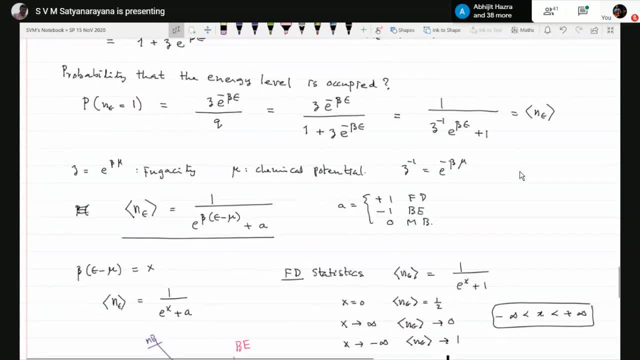 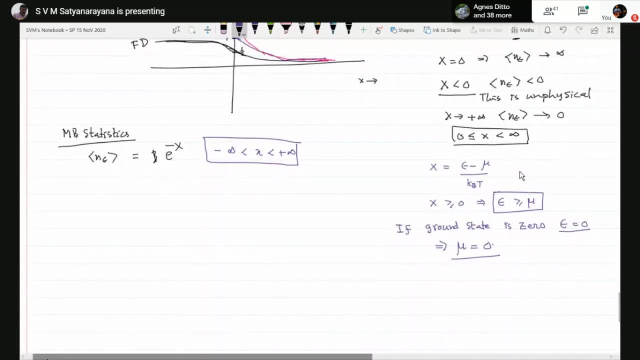 We will also. we can see here the inverse: 1 over m divided by te, by So trajectorially, that of a very big difference. So this is as far as the occupancy numbers are concerned. Now we can talk about general, For example, one of the important things in any system is to 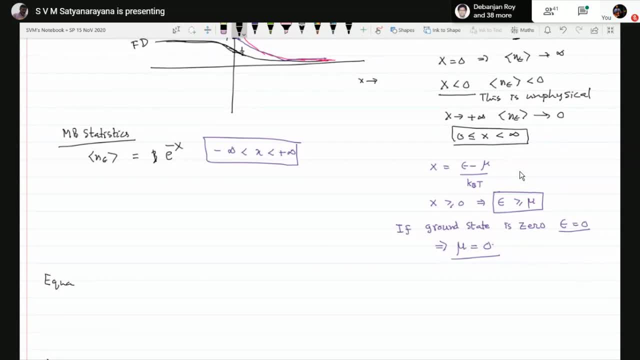 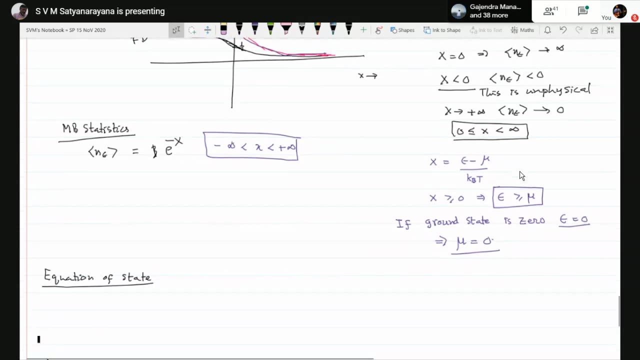 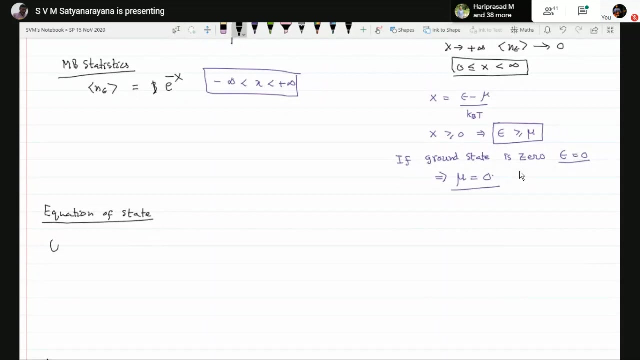 talk about equation of space. So the basic idea is same thing, like what we discussed when we talked about branch and unbranched space. So we have this: we have q for f, t plus product over j, 1 plus z, e to the minus. I can simply write it: the product over epsilon. 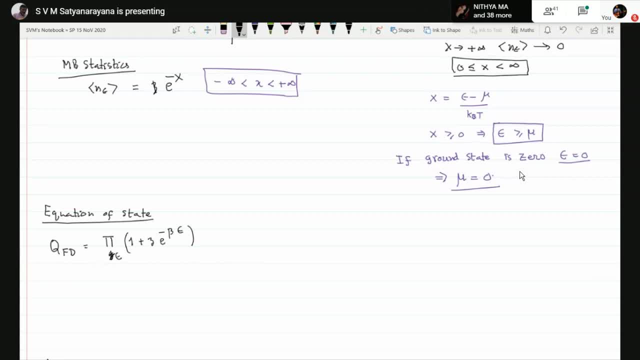 into 1 plus z into beta. This is product over all single particle, product over single particle. And this implies I can write down the p, v by k, v, t as logarithmic, So I can write down the question over here. So let us take a look at this formula. So if we just spend 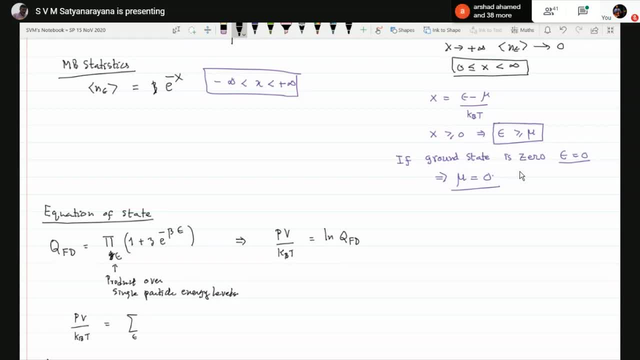 the energy equal to u f t plus u f t, p v t plus 1 plus z, e to the minus beta. So let us take a look at this. So this is a solution. So this is e to the minus. this is a equation. 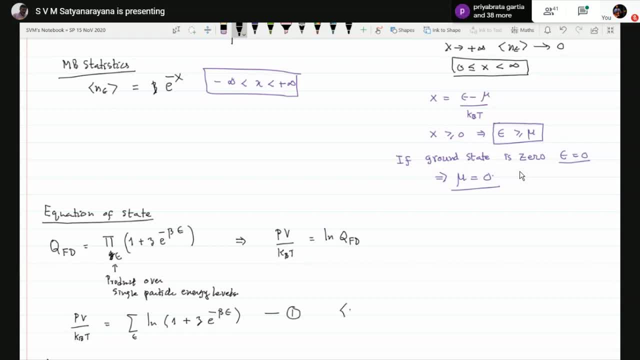 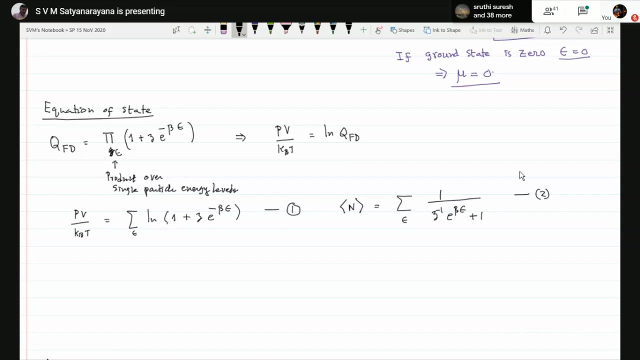 one. And then we have equation 2, namely the n, the average number of particles is sum over epsilon 1, pi z inverse e to the beta epsilon plus 1, this is equation 2.. So I can state it easily. so we can state: eliminate z between equations. 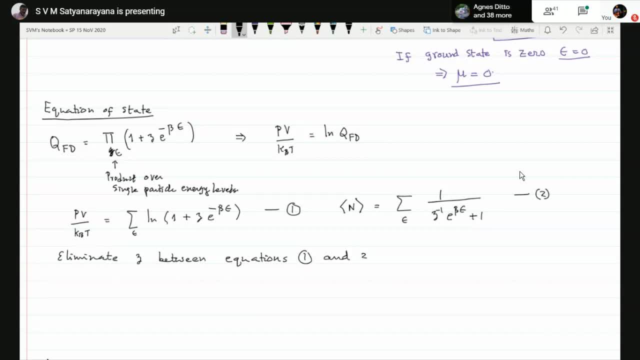 1 and 2.. So to get the equation of state. So as long as I do not have to find the equation of state, I can make this statement. But finding the equation of state by doing this elimination of z is not very easy because it is. it is not very easy because this has some over all. 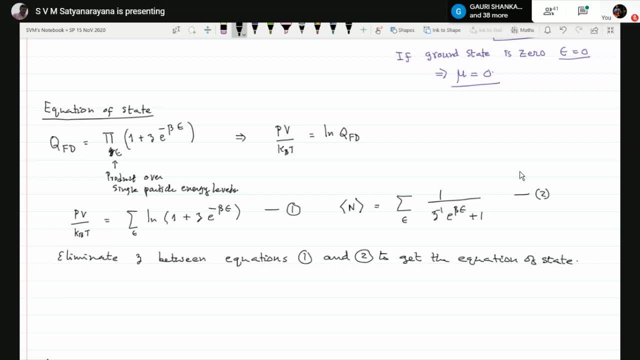 possible states with so many terms, in fact infinite sums on both sides. So what one generally does is that you try to, for example: so it is not easy, So please understand that it is not. it is not easy to do this, So one can do this, one can do this, one can do this. So 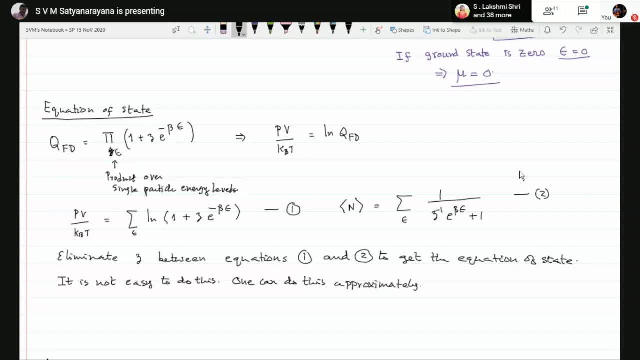 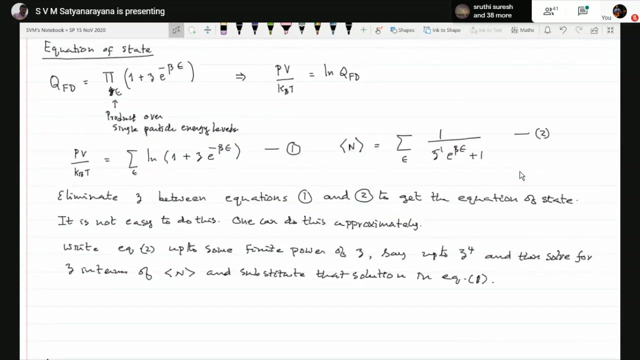 approximately right. please some uh, equation, finite power, finite power of that, and then solve for. solve for in terms of, in terms of, and substitute- wicked Termination. that is solution question 1. then you will get an equation of state which is now so. this is the procedure and the the same procedure can be used. 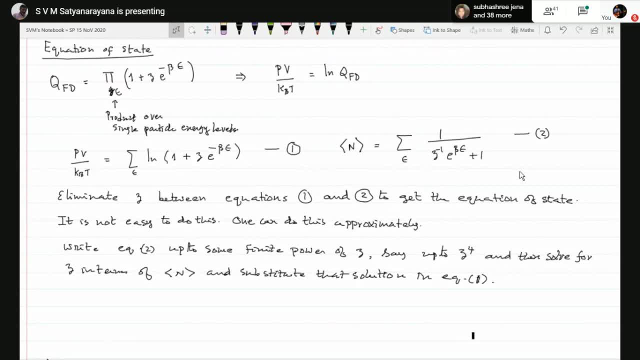 for finding the equation of stateava. So this is something which, but when we did the ideal gas using the grand canonical ensemble, I demonstrated ideal gas by eliminating z. z can be eliminated very easily in that whereas in a general case one has- in fact people try to do this using Mathematica kind of software. 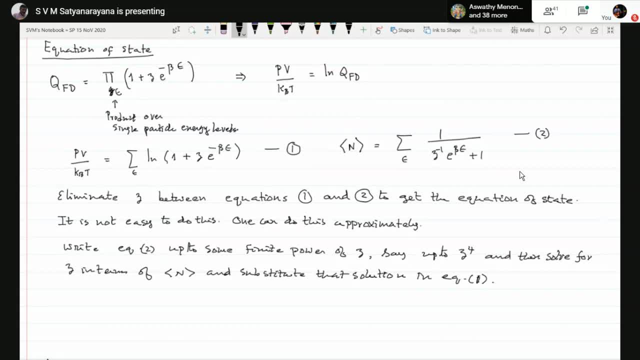 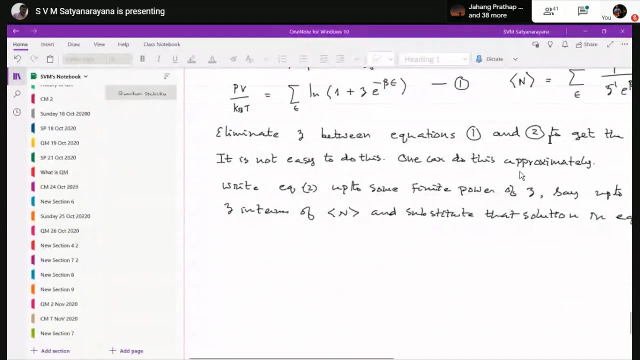 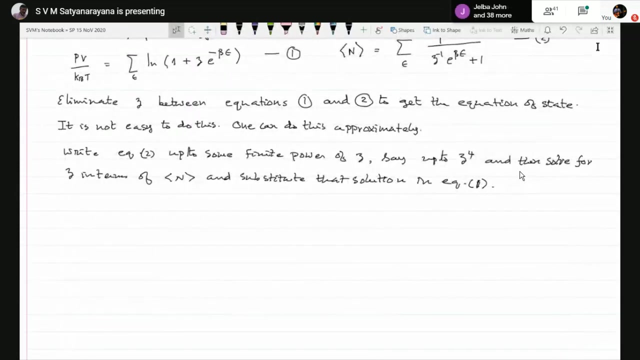 where you can invert one relation, find z as a function of n and substitute that. So we have expressions that are kind of almost completed, the foundation of the quantum statistical mechanics. Now we have to see what are the things that we are going to do in quantum. 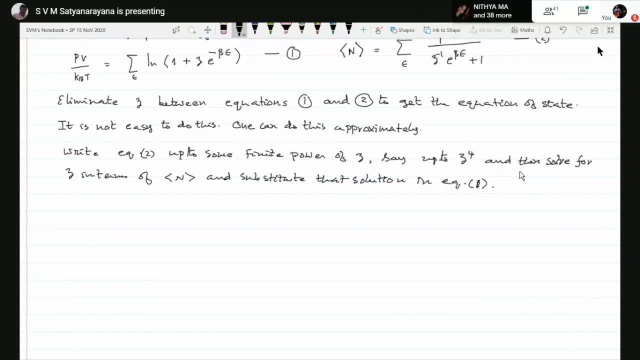 statistics. So, as I told you that we have two types of statistics: In the Bose Einstein statistics. So in Bose Einstein statistics, we are going to look at the work of Bose Bose work. So we are going to look at the work of Bose Bose work. 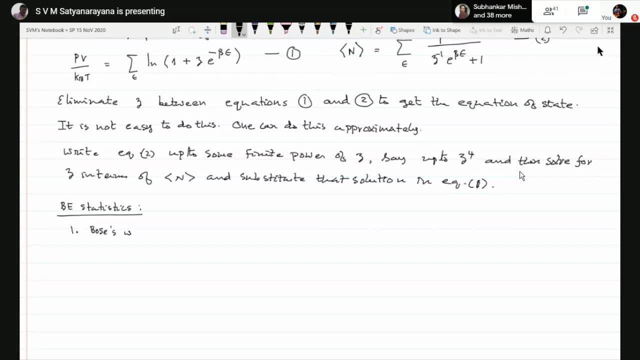 Thank you, Thank you, Thank you. This is work. work is developed and, due to function, goes to on, So we will try to understand how he his idea of, in fact, the issue of identical particles which now learn as a consequence of the symmetry properties of the wave function, was introduced. 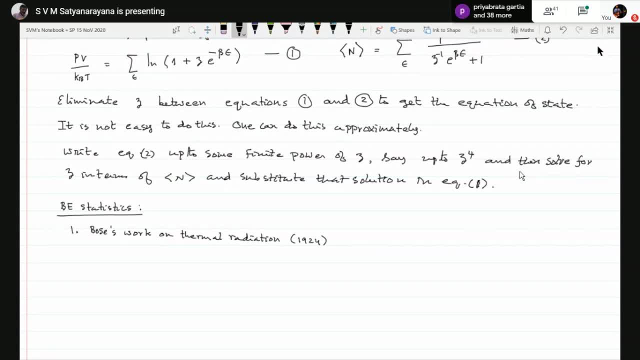 in a very innovative way into this statistics by Bose, even before the wave function exercise was discovered. So we will look at the work of Bose in terms of thermal radiation And let us also try to do it in some detail so that they get a hand of the essential insights. 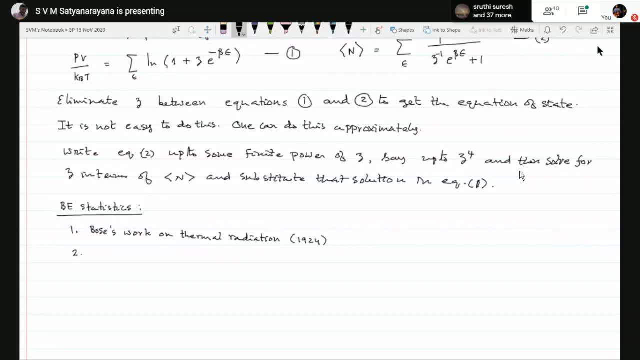 into the work. And the second application that we will look at is what is called Bose Einstein condensers. This is an important, an important feature of bosons, which we will look at in a very detailed way. This happens for particles with finite mass. 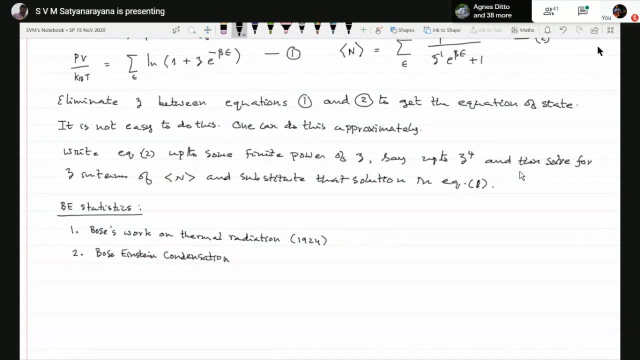 And Bose Einstein condensation is a macroscopic occupancy of a single particle ground state. So this is something which is very unique to bosons and Bose Einstein condensation. And the third application is we will copy of a particle with finite mass, So we will look at it in a very detailed way. 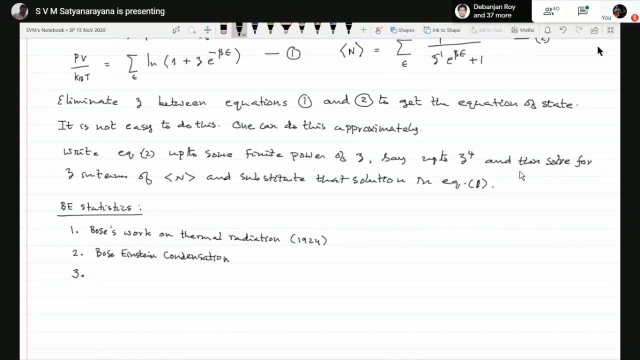 This is a material based on your seismology. Thank you very much, Thanks very much. Thank you very much. do these three things for sure and if there is time, then we will try to look at superfluid helium and certain excitations. 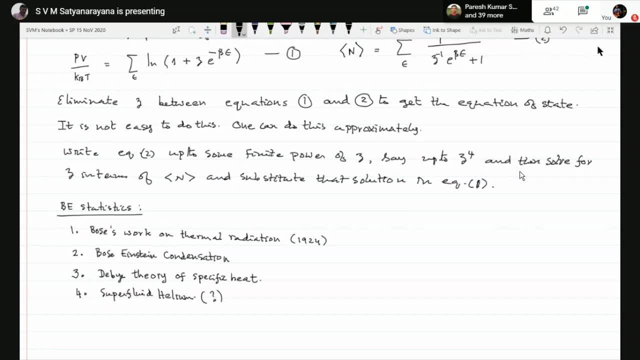 but i will just keep it not very sure. if we can reach, if you are able to do it quickly, then we can. and then let's go to fd statistics. uh, in fd statistics we have. so we will first talk about electrons in metals, in metals, and we discuss various physical properties. 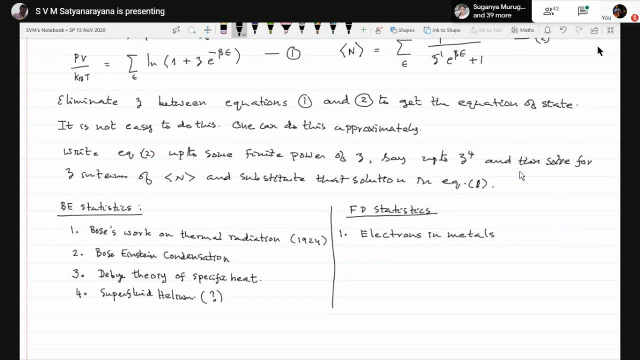 such as specific heat of electrons. classically it was supposed to be temperature. independent experiment showed that it caves linearly with the temperature and we show that use of thermodynamics statistics brings that feature back in, compared to a drug-laden theory in classical physics. then we have, uh, two theories of magnetism. 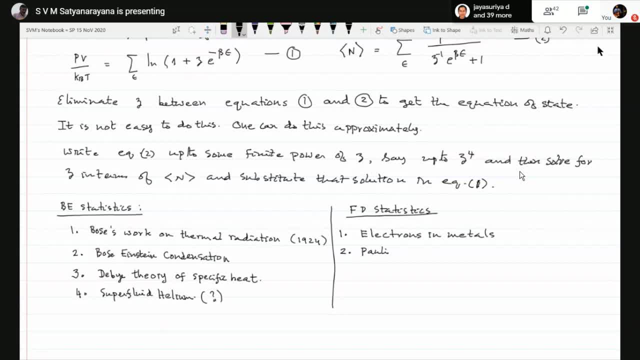 it is called Pauli theory of paramagnetism. it is called Pauli theory of paramagnetism. then there is Lando theory of diamagnetism. then there is Lando theory of diamagnetism, And then we have an application that is quite different from what we have seen so far. 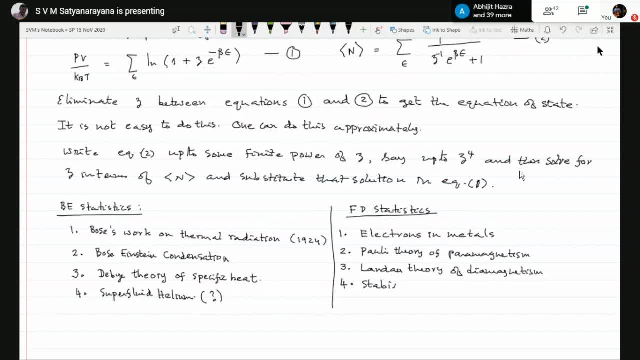 Namely, we will talk about stability of whiteboard stack. This is also an application of the stability of whiteboard. So this work is initially was done by Chandrasekhar and we see how, as an application of Fermi-Dirac statistics. 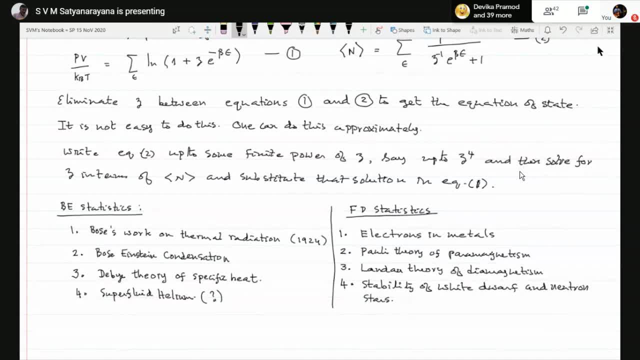 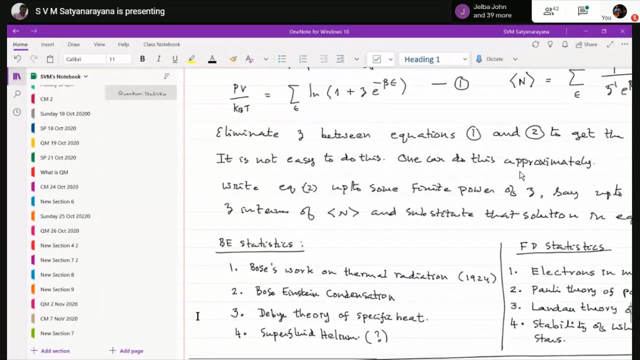 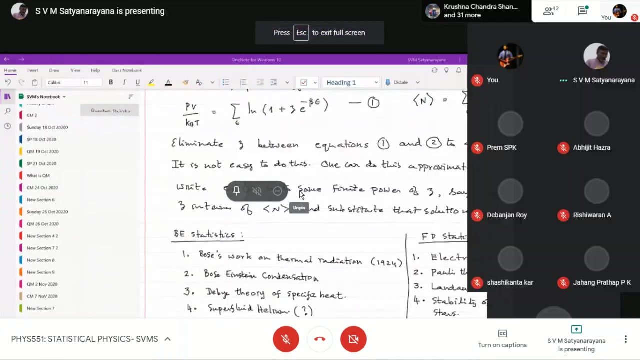 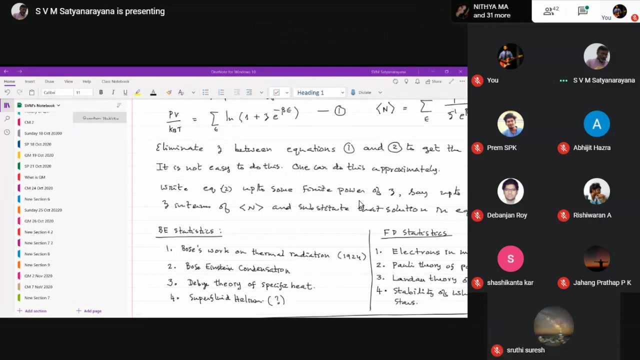 the Chandrasekhar limit can be derived. So these are the applications of Fermi-Dirac statistics. So these are the topics that we will cover in this unit as an application of our products. Okay, I will stop here and set. 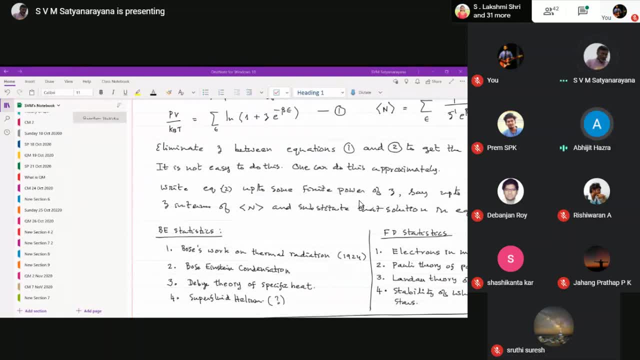 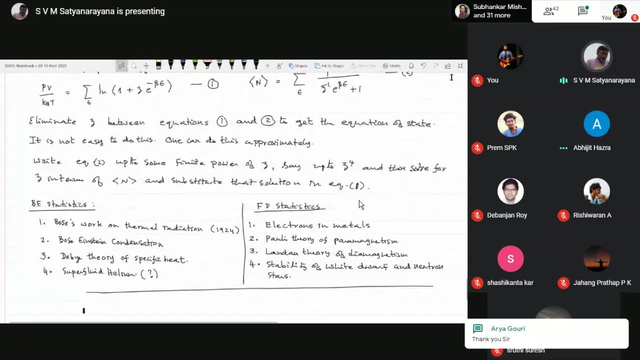 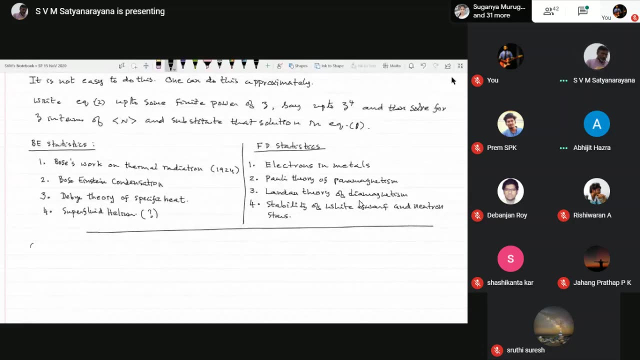 Okay, Yes, Sir, are you going to study more applications of grand canonical partisan function? Yes, Like quantum one? Yes, So I am going to do two applications. Okay, so, in grand canonical ensemble. So there are going to be two applications. 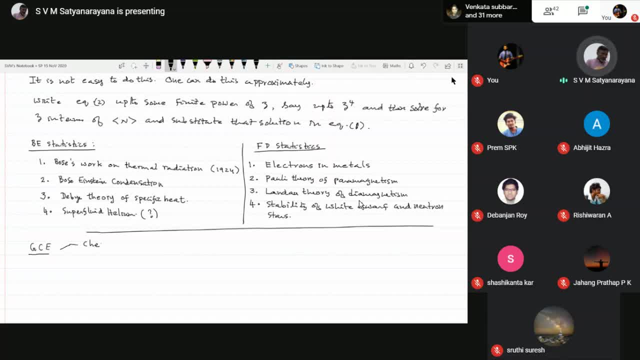 One is in terms of chemical reaction. Okay, based on how actually you are going to calculate rate of chemical reactions from the grand canonical partition function. So this is one application. The second application is: it is also related to this, but it is also related to some biological. 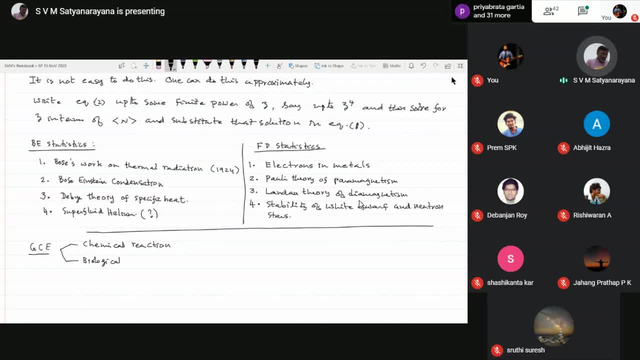 It is a single application. I will talk about it later. So, biological phenomena: With respect to one or two phenomena of biological sciences, I will try to show how, using grand canonical ensemble, one can. So these are the two applications which I will do.